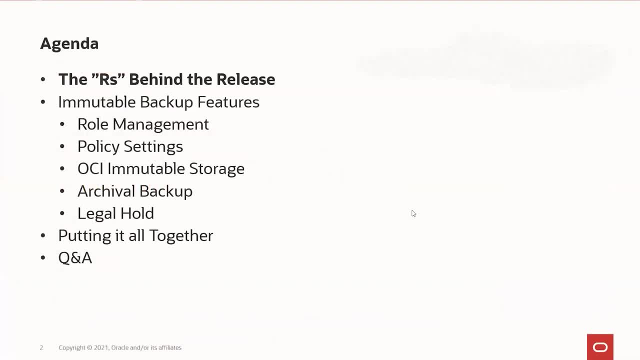 Thank you. So here's the agenda. We're going to briefly cover what is actually the main drivers behind this latest release, And so then we're going to cover most of the quintessential features that are comprising this 21.1 release, including commutable backup features. 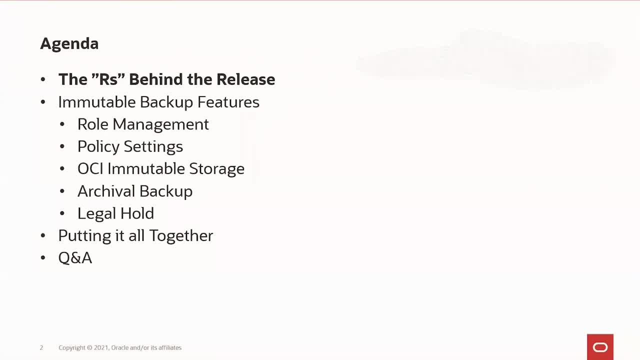 We're going to touch on the role management changes. So we're going to talk about new policy settings. I'm going to start talking about immutable storage and regulations and compliancy in respect to the new policy. We're going to touch on the role management changes in respect of the enablement of the compliance regulations that start with immutability. 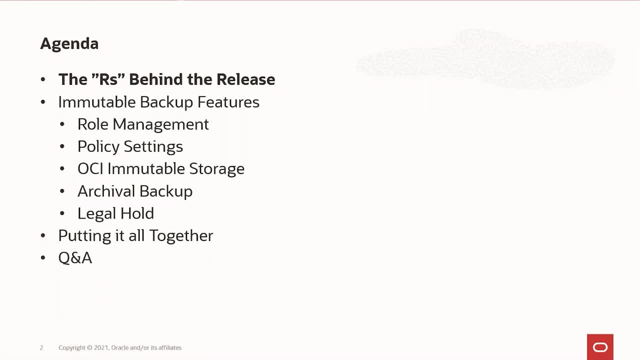 And we're going to touch on the additional features related to the archiving, backup, and also new set of the features related again to the compliance is called legal hold. And then we're going to wrap it up with kind of compelling picture just to put it all together and just to show the complete picture in respect of the overall evolution of the recovery appliances. 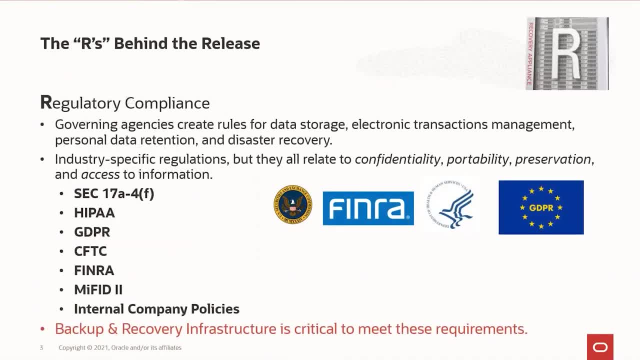 So there are two major R's behind this release. So number one is, as I mentioned, regulatory compliance. You, of course, are well aware that different verticals have different compliance regulations, like, for example, SSC 17A, related to the financial vertical, that will have HIPAA regulations. 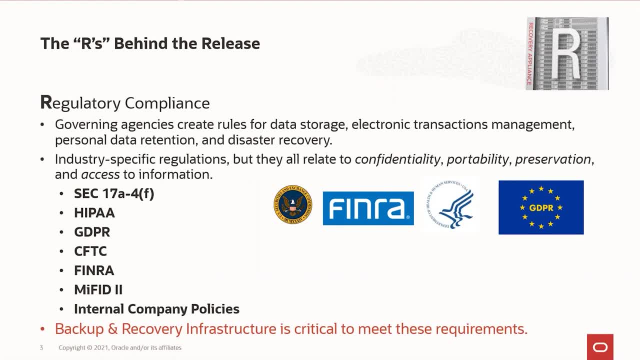 So for the health care, we have GDPR for European entities And what is really important, that's the backup and recovery infrastructure is pretty much the carrier, in a sense, of the execution of this backup and recovery regulatory compliance. So, for example, HIPAA regulations demand that you're going to be able to retain every record for seven years. 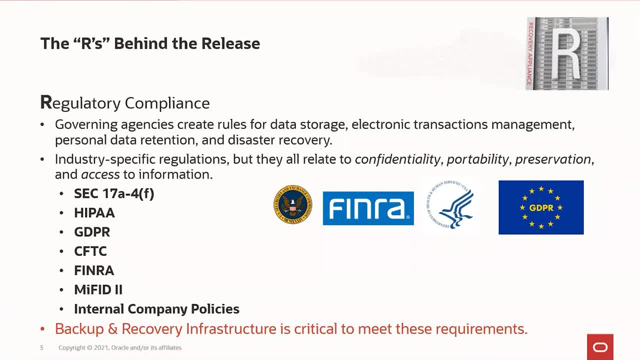 SSC. depending on the financial institutions, they have their own regulatory compliance that actually dictating not just the quality of the storage and application driving the storage qualities, but also demanding specific number of copies being retained. And so when you're looking at the regulatory compliance, they enable itself for the archival, et cetera, et cetera, et cetera. 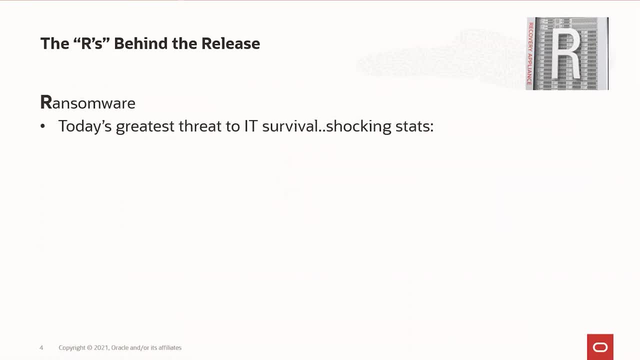 So the second one is ransomware, And even though that it might not necessarily be related to the compliance, I will explain later on that actually both are extremely cross-linked And so obviously the ransomware today is the greatest threat to the IT survival, because it just brought new, additional challenges. 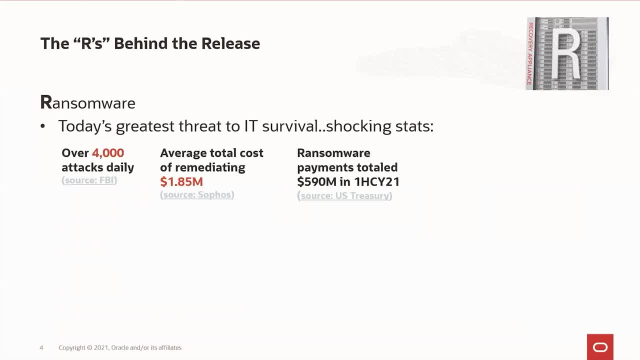 challenges And the overall outcome of the ransomware threats. we have over 4,000 tests daily. We have average cost of the remediating close to 2 million per attack. Ransomware payment totaled over half a billion just in the first half of the 21.. But to me the most. 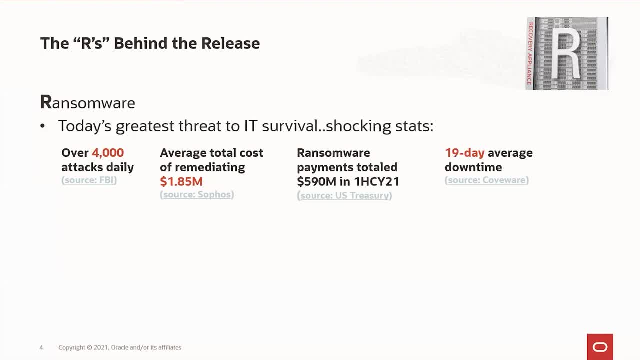 critical failure is the 19-day average downtime that has been reported. If you're going to take a look at the previous screen, it easily can be stated that 19-day average downtime is much more expensive than all of the three buckets in Radovitz combined, For example. 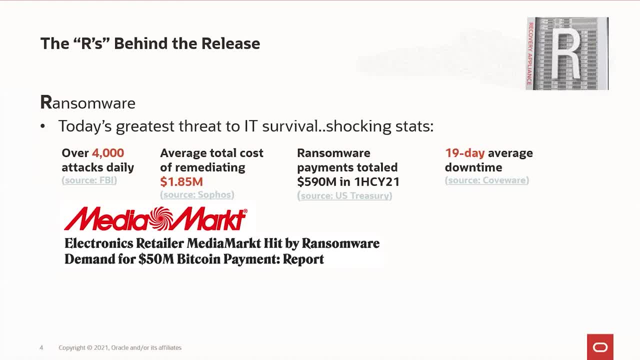 one of the latest attacks on the media market, which is pretty much identical to the Best Buy retail in Europe. they face demand for the 15 million Bitcoin payments And the problem is not just the payment itself. The problem is that how can you ensure that the payment? 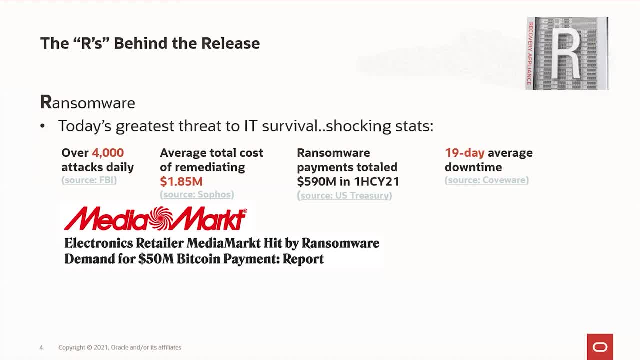 is not just the payment itself, but the payment itself. And the problem is that how can you ensure that you actually going to be able to recover? Because even though that you might pay ransom, even though that you might get back your keys, it's not necessarily that. 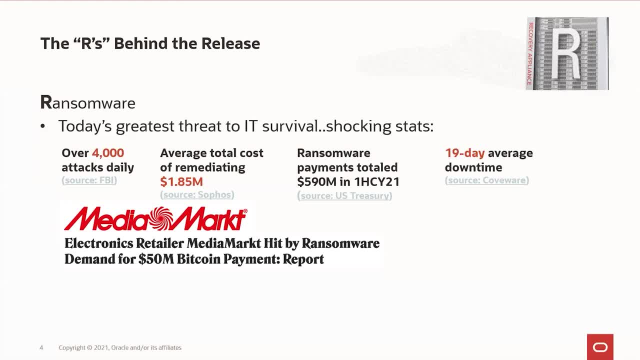 your infrastructure is still not being affected or still not being compromised by the attack itself And this is why we say that the backup and recovery infrastructure today is the last line of defense. And if you're going to go back to the regulatory compliance and if 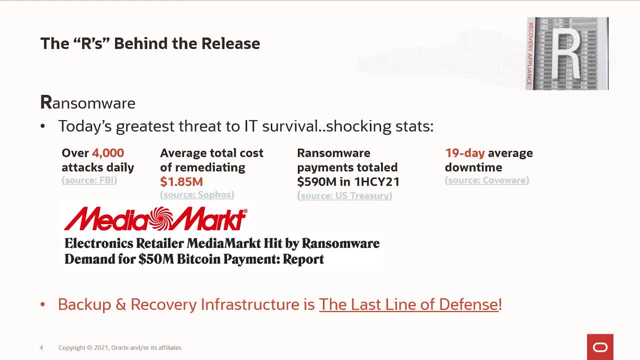 you're going to go to the disaster recovery practices. it's basically the same thing. Basically, all of these factors are easily translated into the ransomware prevention. because if you do not follow just the basic rules, if you're not really in control of the 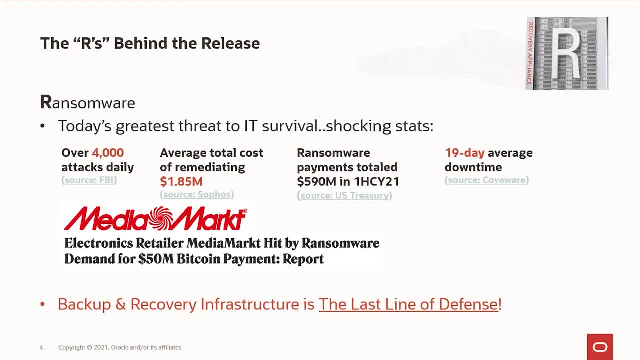 last line of defense, most likely you're going to have to surrender, And so what is really important about this is that ransomware is not successful unless it's going to be compromised in all of the, including the last line of defense, And if you can ensure that this last line of defense is pretty 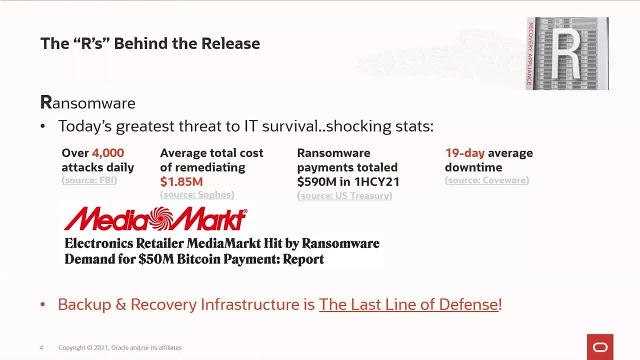 much the same, then you're going to have to surrender, And so what is really important about this is that ransomware is not successful unless it's going to be compromised in all of the impossible to touch. then you win, and most likely you're going to be prevailing in a sense of 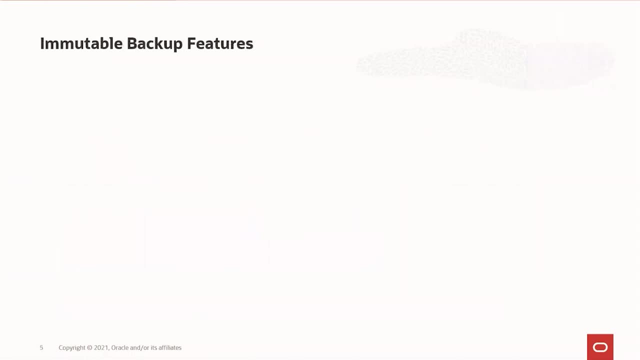 facing ransomware attacks. So let's talk about some new features, and we're going to start with immutability. And it is really important to understand that, even though that's a lot of vendors claim that they have immutable features, the essence of immutability is not just the 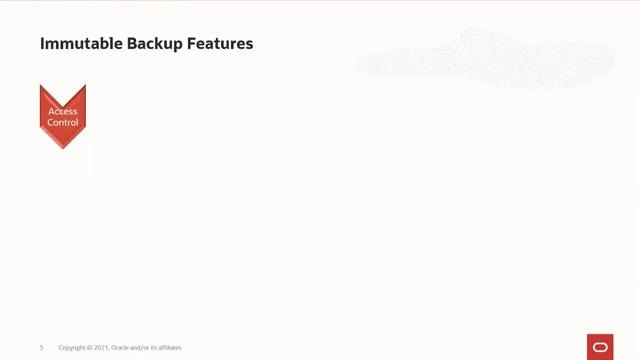 storage quality, So we're going to talk about it in just a second. It's actually a solution, And to have a compelling solution you have to deliver a lot of critical qualities that go just way beyond immutability of the file system or something. 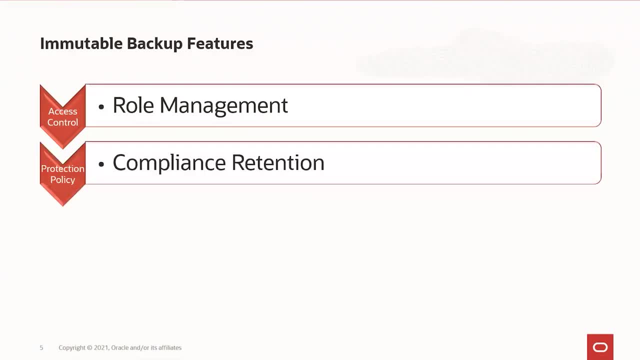 like that. It includes role management, It includes compliance retention, in a sense of the protection policy. It includes archiving, because obviously backups only last that long And if you're going to be talking about the real last line of defense, obviously you have to make sure that your archive. has the same quality as the file system. So you have to make sure that you have the same quality as the file system. So you're going to have to make sure that you have the same quality as the file system. So you have to make sure that you have the same quality as the file system. So 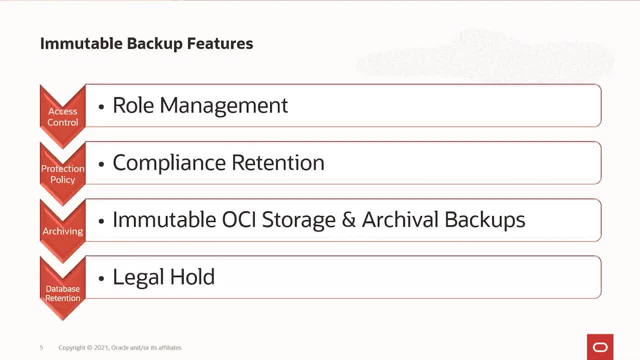 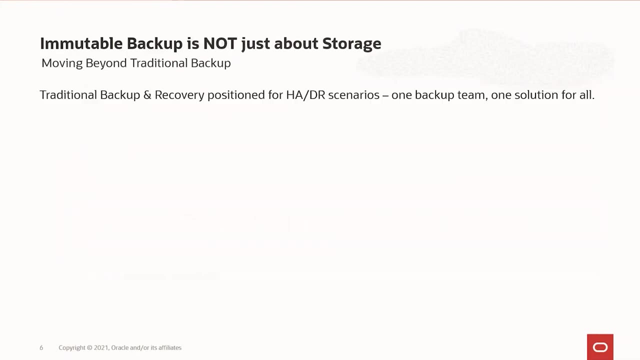 the immutability, just like the backups And, last but not least, legal hold, and so I will explain what is really important for the immutability and compliance going forward in respect of the legal hold features. So let's start back talking about the immutability and just making the level set. 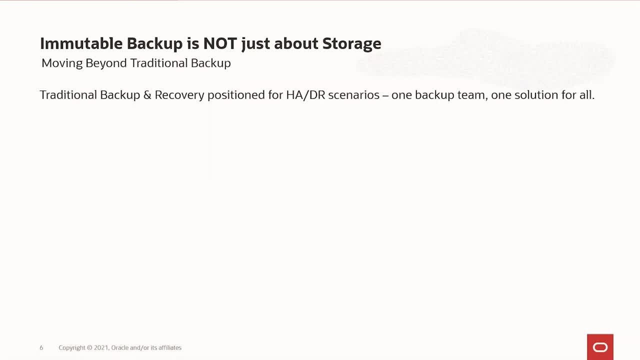 What does immutability mean? because, like I said, in a lot of cases different vendors. they basically develop and elaborate on the immutability in absolutely different flavors And in our case we want to make sure that the solution for immutability targeting regulatory compliance and complete ransomware prevention. 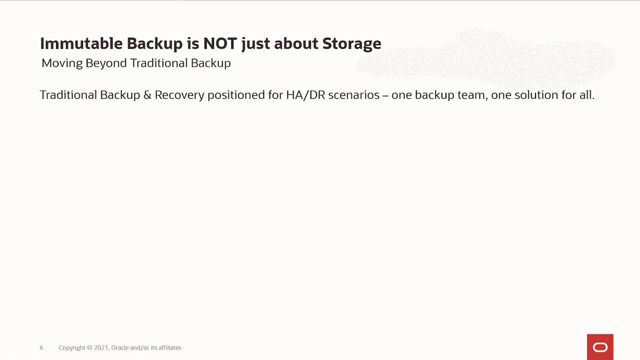 includes not just the typical immutability qualities for storage vendors like, for example, Dell, EMC or Cohesity or Rubrix, And it's not just addressing KTDR scenarios, because the problem with the legacy frameworks and the problem with just immutable file systems developed by different 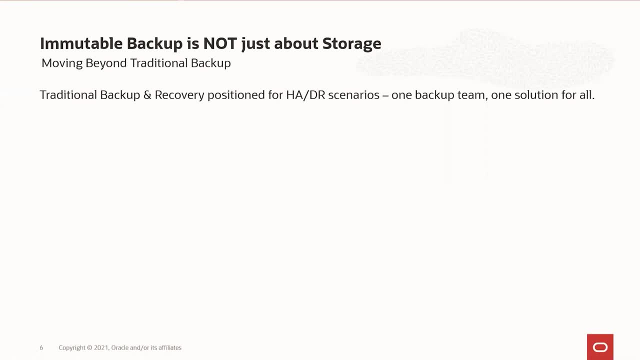 storage vendors. they still have the same huge hole. It is one team that actually has access to the kingdom and if this team is being compromised, most likely you will never succeed in the sense of the recovery. And this is what we're talking about, so that it creates the single point of failure, Because 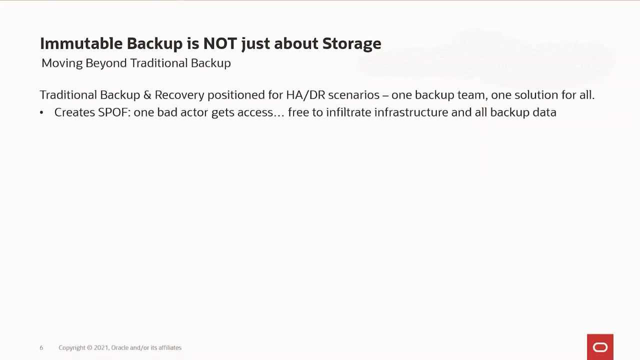 again one bad factor: being compromised most likely is going to be capable of compromising your entire infrastructure and backup data in the same time. So back to the kind of definition of the ransomware. then So the relevancy of the last time of defense. They start from the. 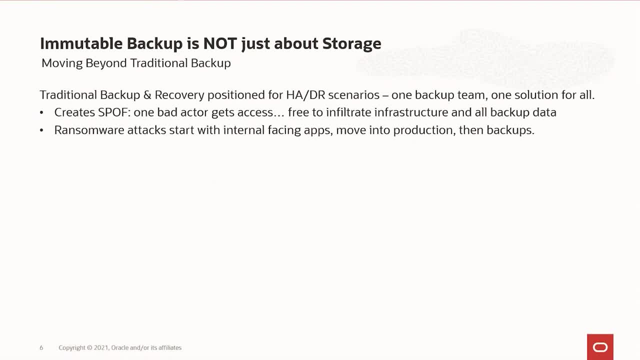 application penetrating into the production infrastructure and then penetrating the backup infrastructure And the typical legacy deployments most likely face extremely hard challenges, not just in the respect of the compromising and that single actor, but also because of the traditional storage quality. So, like persistent connections, most likely you will not be able to prevent complete 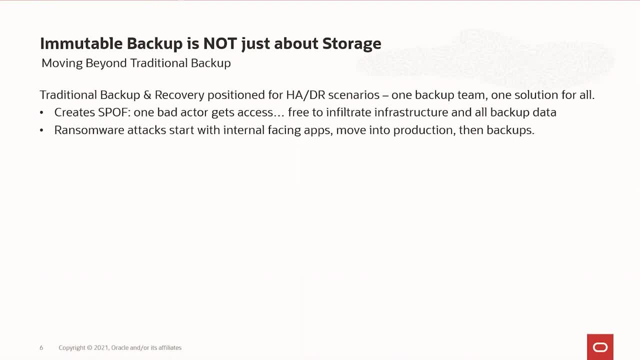 basically just damage to the both primary and secondary infrastructures. So let's talk about backup data. So, when we started talking about, the backup data should be holistic and protected against malicious deletion modification. Again, this is not just of this- the storage quality, As you can imagine that if I have access to my critical data, 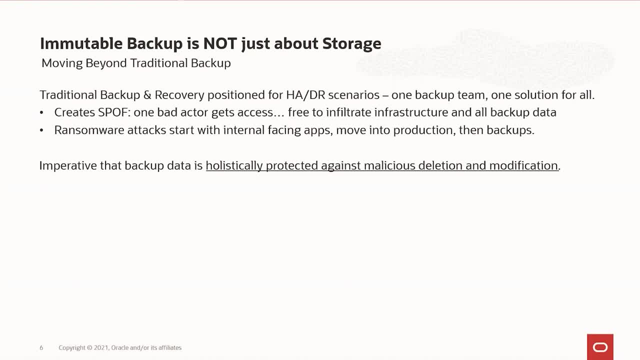 most likely. even though that's you might have immutable storage somewhere in place, it doesn't mean that it's not going to be compromised. So immutable backups: in our case, we target adding yet another layer of protection, And so we will talk in just a minute, probably, about backup costs. 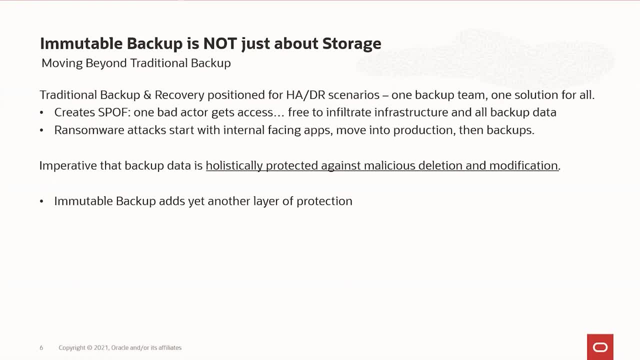 a short couple of minutes. just what do we mean by providing full immutability? The one thing that's worth mentioning is overall evolution of IntelliTouch. in just a second, The evolution of the immutability went a long way, from where it was incepted and to where 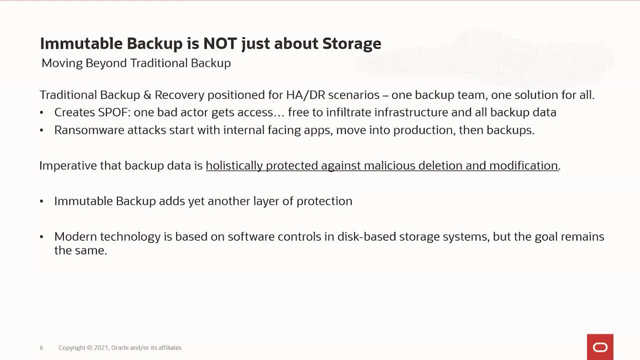 it stands today just because of the evolution of the storage system, because of the evolution of the overall IT infrastructure. So today we have absolutely different conversation about what does it mean to have complete, bulletproof immutability? And the definition of the immutable backups in traditional way is that so backups can be deleted or modified until 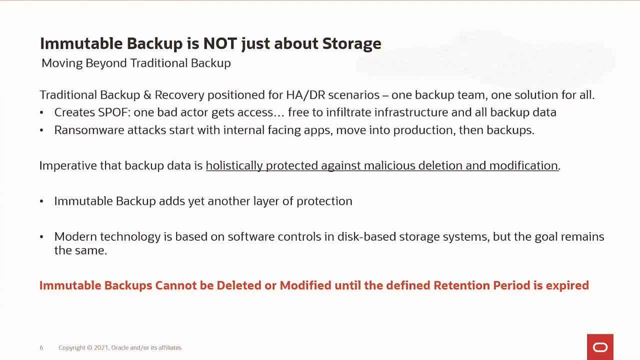 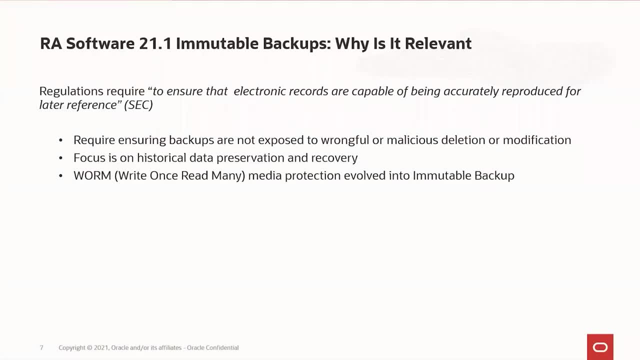 defined rotation period is expired or forever. So why is it relevant to the conversation? If we will take a look at the definition of the requirements for the regulations, let's say specifically SSA regulations for the financial vertical, it requires to ensure that the electronic records are capable of being accurately reproduced for later reference. 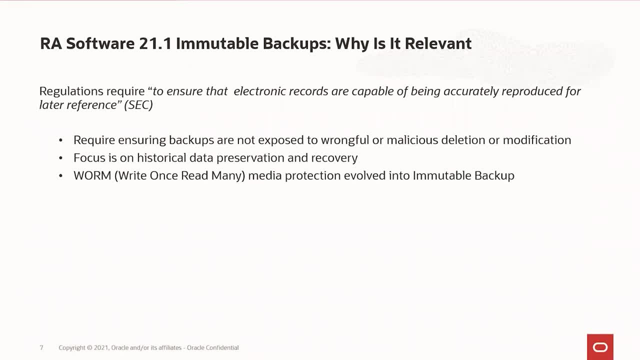 And it all started some decades ago, of course, and so the first company that's actually dealt with the typical cloud services for this type of the situation, of course, is Siren Mountain. Everybody was doing tape outs, everybody was doing warm tape outs, everybody was. 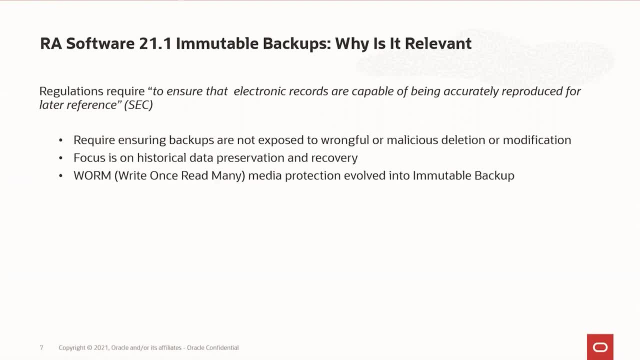 making sure that. so they got to be keeping all of the data that was available in the off-site storage And the focus always been on the historical data preservation, recovery and as a response to the compliance regulations requirements, And the off-site tape outs were targeting to ensure that backups are not exposed. 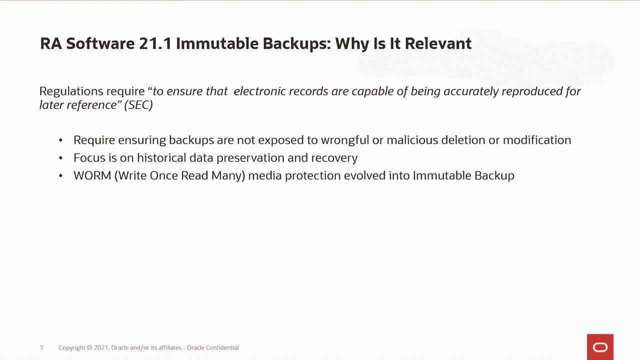 because Iron Mountain- basically that was a part of the contract obligations. they had to make sure that the warm tape outs are not going to be compromised or attached by anybody else. And ransomware now introduced new challenges. but solutions are all the same because you still have to ensure that compliance modes with immutability for backup storage is going to. 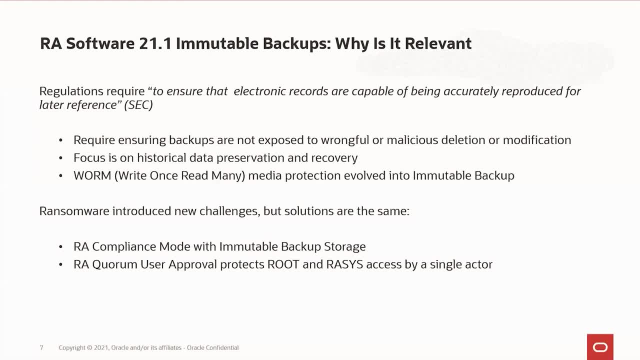 be fully maintained. So you have to make sure that, in a sense of the admin access is not going to be creating a situation when you have a single backup. You have to make sure that you have a single actor that might be capable of accessing truth and 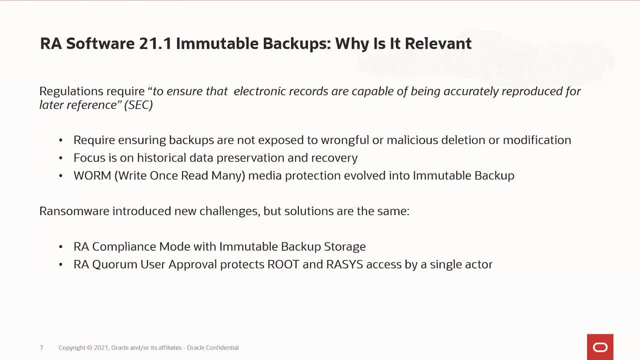 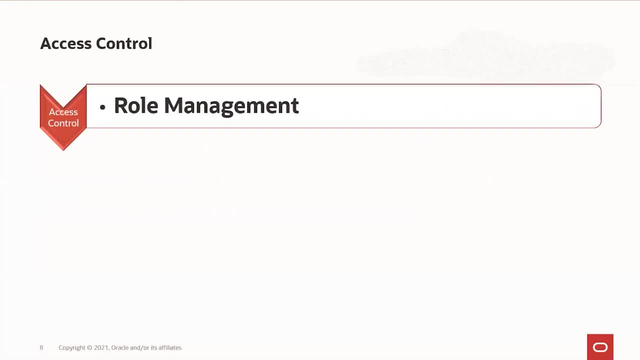 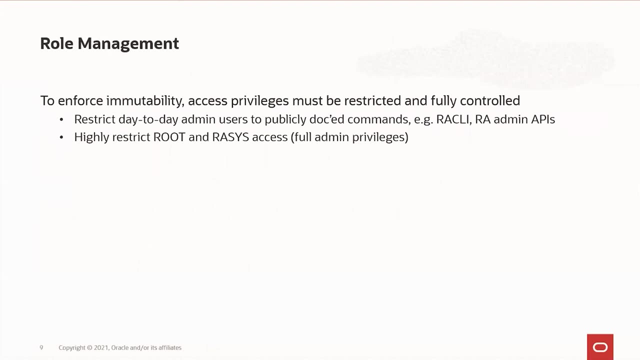 racist credentials for the Oracle databases. So, starting with the role management, we are talking about some new controls that were introduced, So just make sure that we're on the same page here. All these changes are only related to the compliance mode for the recovery plans. 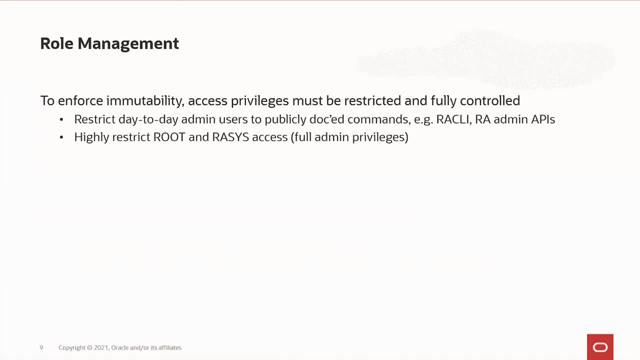 If you do not want to deploy or for whatever reason you cannot deploy in your environment the specific mode that is, targeting, immutability and compliance mode. it doesn't mean that you have to enable this, But we give you a choice now. We basically walk away from the models related to the 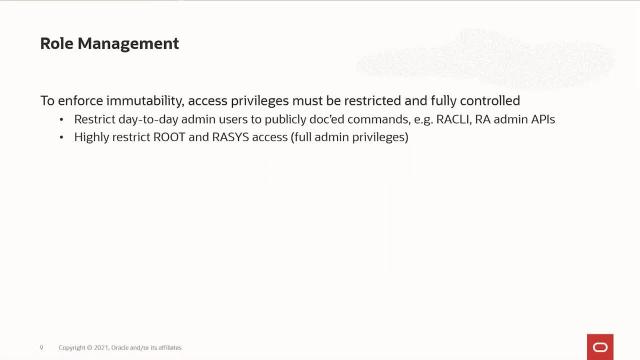 full admin privileges for the routes and the RACs, Meaning that we want to restrict day-to-day admin users to just the public and documented commands and to shut down this extremely critical access to your systems, just to ensure that your system will never be compromised by the RAC actor. 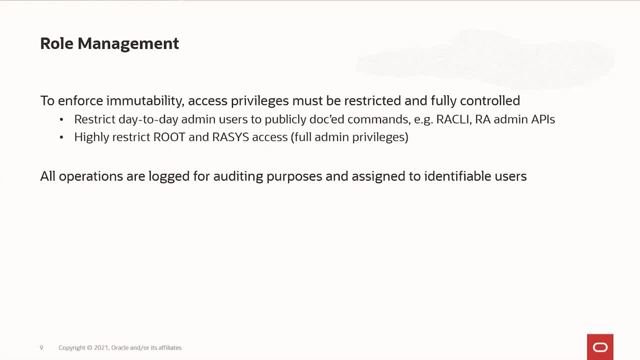 One of the things that are demanded by the compliance regulations is that all the operations should be locked and also should be mapped to the identical users, So if something is happening, you're going to have access to the forensic evidence identifying who might be the wrong actor on your 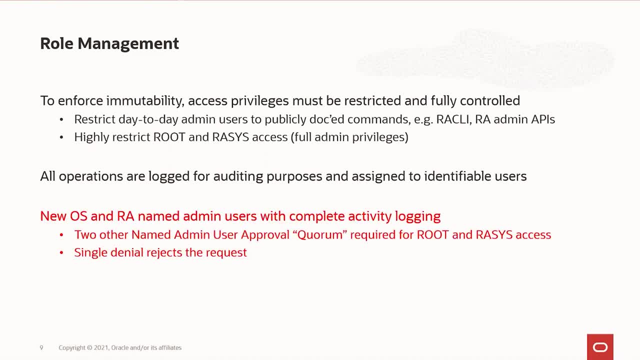 team trying to do something crazy, So new OS and RA named admin users with a complete activity login were created. We have now the model that we call Quorum, And so Quorum means that if you want to have access to the route, privileges the other. 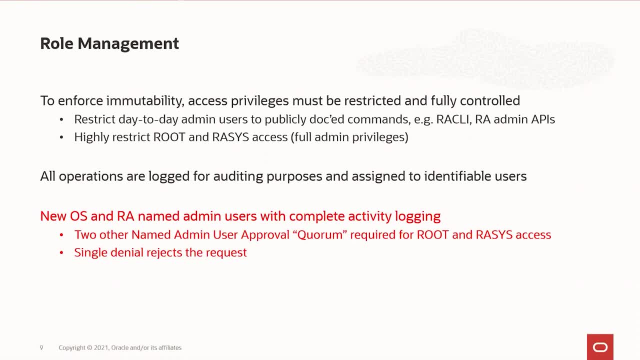 members of your team are going to be notified with a request to grant access to the RACs And if, for whatever reason, at least one of them will not be willing to grant you the access, the access overall is going to be denied. So it is critical because, again, you never know. 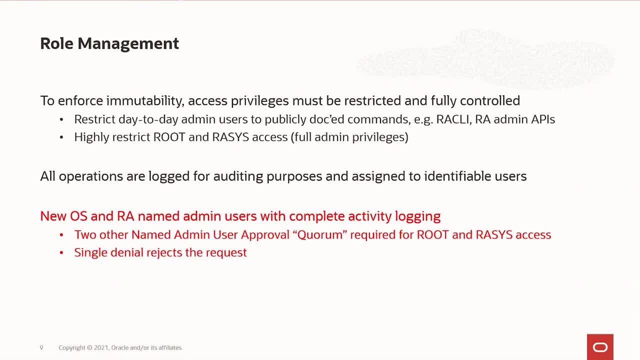 how many team members might be compromised during the ransomware effect. But at least it gives you some peace of mind that you can build new practices around these type of the log and enroll management in your environment to ensure that if something crazy is happening, you're always going to be ready- Compliance retention. So, as you might notice, 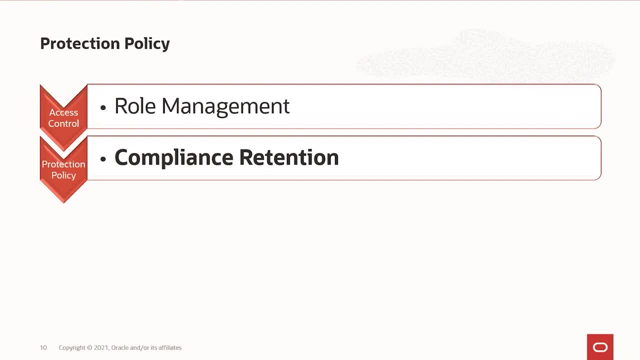 we introduced a lot of new terminology for the recovery appliances with this release, And so this is just quite a session just to make sure that you have a complete picture and complete understanding of why did we do this and what are the ramifications, in a sense, of the recovery appliance deployments and configuration going forward. 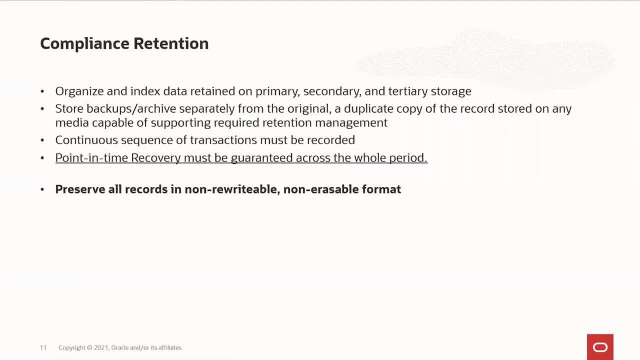 So one of them is compliance retention. So what does mean compliance retention From the kind of 10,000 feet view? the compliance retention has always been targeting not just the active environment but also passive environment, meaning that you have to have access and complete set of the catalog information to access your 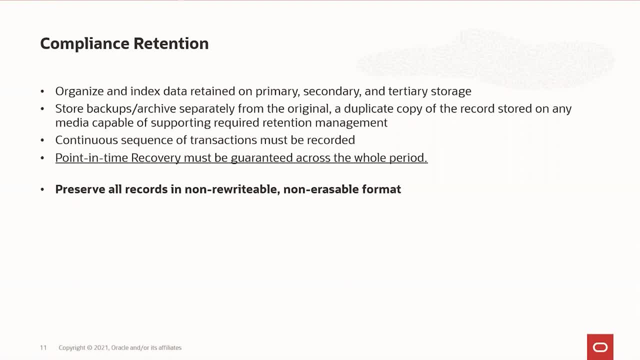 primary, secondary and tertiary storage. And it is important because if one of the tiers is not compliant, you don't have overall compliance to start with. So in a sense we just carried over this type of the requirements to the recovery appliance And we're just trying to make sure. 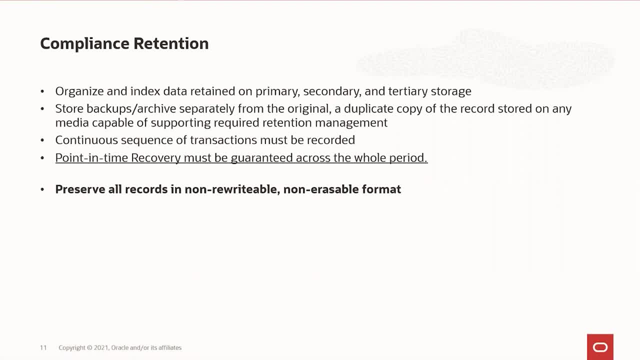 that's going forward. So we got to be basically fit in the mold And one of the important factors that's in any compliance model is compliance retention. So if you have a complex environment mode by the recovery appliances, you're going to be able to have access to the point-in-time. 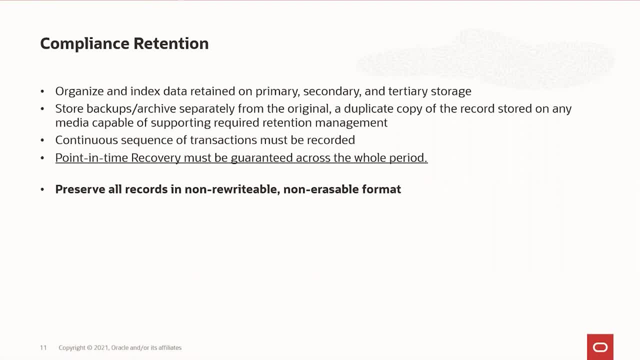 recovery. Why? Because it's also related to the same compliance and legal obligations that you have in your environment. Comes tomorrow, legal, comes to you and wants to have complete access to the specific set of artifacts and you have to produce them as a part of the overall process. 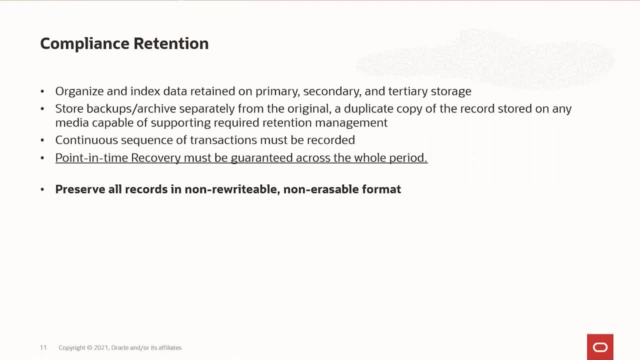 So it all boils down to the preservation of all records in the non-rewritable and non-razor formats as you can imagine. But yet again, I have to repeat it over and over again. this is just not good enough, And 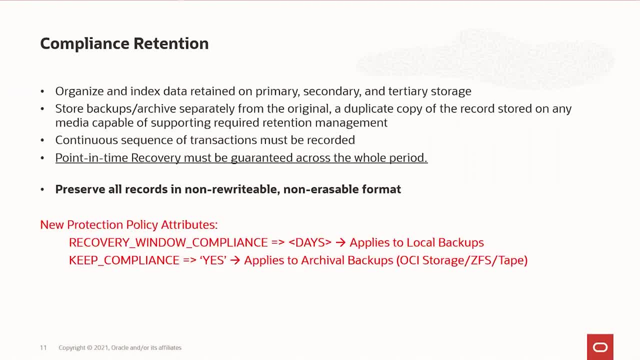 this is just one of the pieces of the huge puzzle, So we have new policy attributes available with this release, So one of them is recovery window, compliance and days Keeping in mind. it applies only to local backups, because anything that is being found out from the recovery appliance. it's not going to be in the recovery appliance. It's going to be in the recovery appliance, And so it's going to be in the recovery appliance. So it's going to be in the recovery appliance, And so it's going to be in the recovery appliance, And so it's. 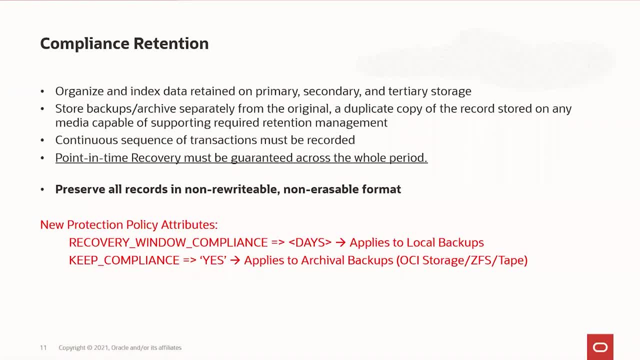 going to be in the recovery appliance, And so it's going to be in the recovery appliance. It's not necessarily non-direct control, Even though that we have a second parameter, emission of compliance. that applies to the backups which are OCI, Sторage, ZFS or tapeout. But even though that we do control catalog. 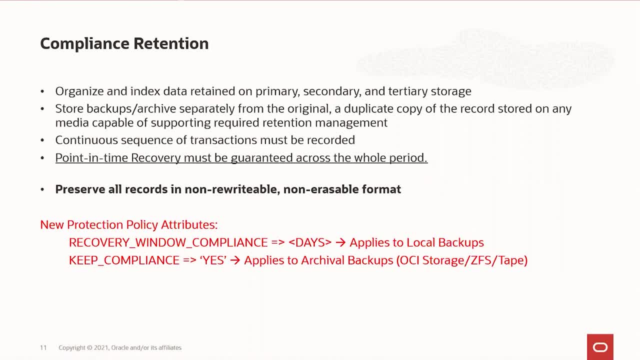 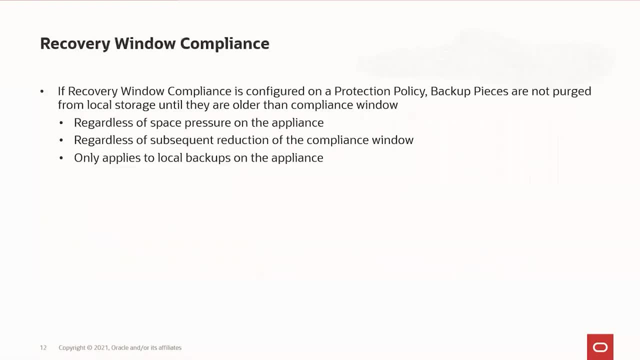 information in our site, it's not necessarily translating into the qualities, especially for the third party vendors, that we simply cannot control outside of our environment. So the second one is recovery window compliance. So recovery window compliance is configured on the protection policy. 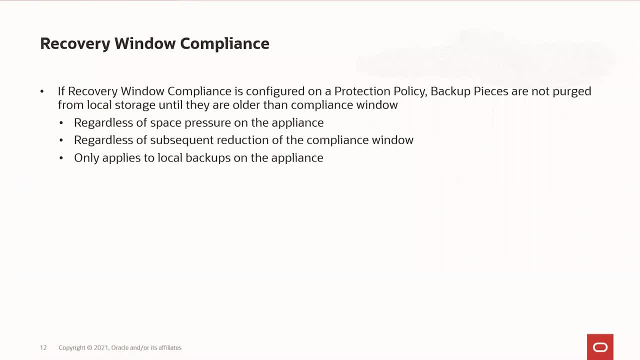 And we are basically preventing any deletion of any data which are sitting within the protection policies with a specific relevance of the window compliance definition. So you might have, for example, a bigger window of the overall backup retention, but it doesn't mean that they cannot be purged. 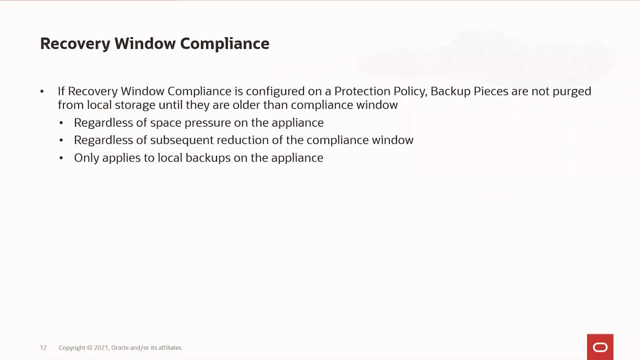 The cases that are within the retention period defined in the window compliance acts in an absolutely different manner. So one of the things that you have to keep in mind starting planning compliance or compliant environments, is that data cannot be purged once window compliance is defined, even in 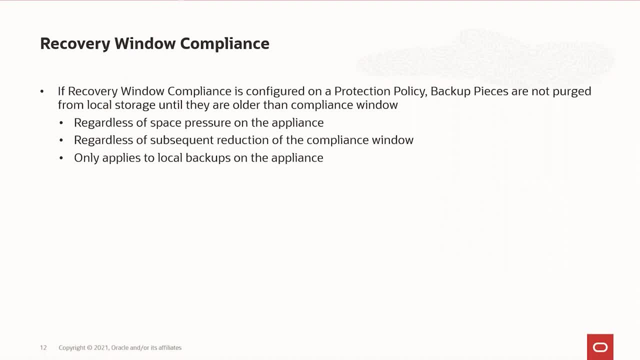 the case of a data breach. So you might have, for example, a bigger window of the overall backup retention, but it doesn't mean that they cannot be purged once window compliance is defined, even in the case of the space pressure, Meaning that the sizing of the environments, even temporary, is going to be pretty much 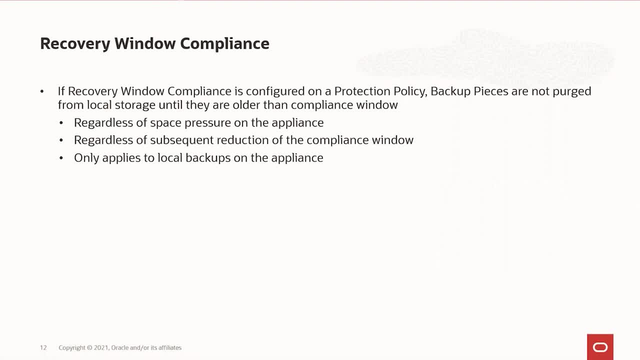 critical. So if you, for example, already kind of filmed the critical edge of the available space, And so you are, and you have to comply and you have to impose the window compliance or your recovery appliances, you just have to size it properly because most likely it's. 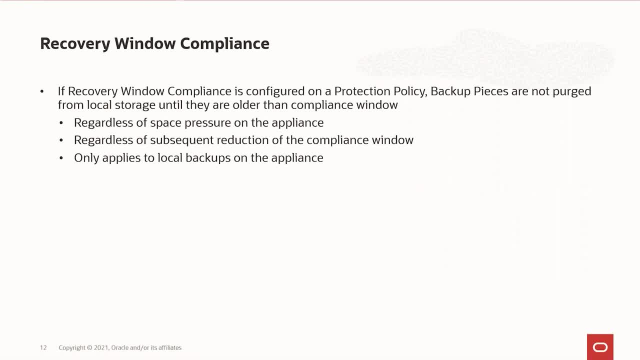 going to be affecting overall sizing and overall consumption planning. The second factor is that you have to ensure that archiving destinations are configured properly. As I mentioned before, it might be out of our control. Even though that we can control the front end, we cannot control the back end. So, one of the cloud destinations, we will mention a number. 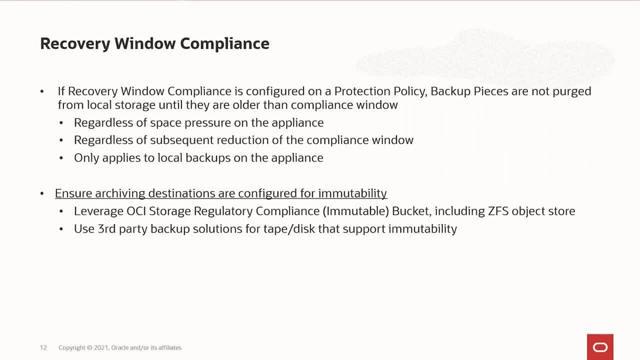 of times going forward is the OCI storage regulatory compliance. There is a special setting that I'm going to show later on the screen how to define the OCI shambles bucket. It is a fully certified bucket provided by the Oracle Cloud Services. It is a good fit and it was certified for pretty much every regulatory compliance regulations. 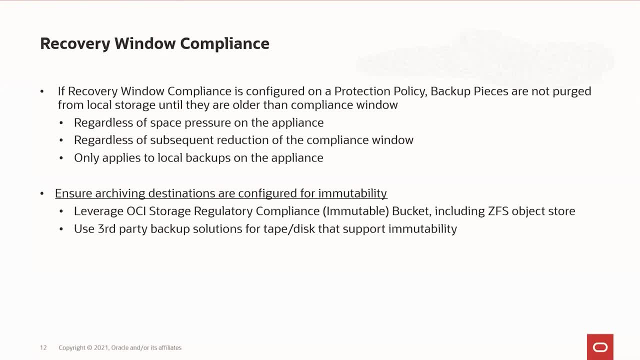 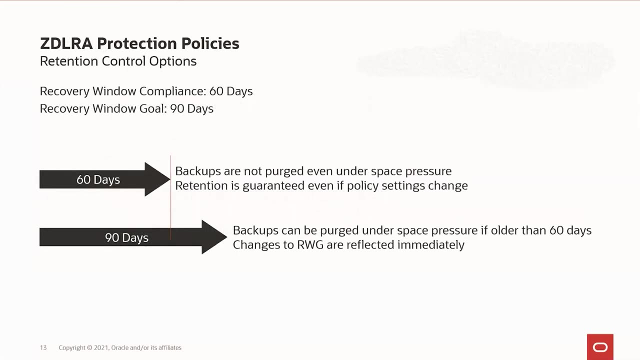 available today on the world market. And the second one that it also includes the EFS object storage. It's also fully compliant and so fully capable of carrying over the requirements. So let's kind of put a little bit of visual aids. How does it all stack up? 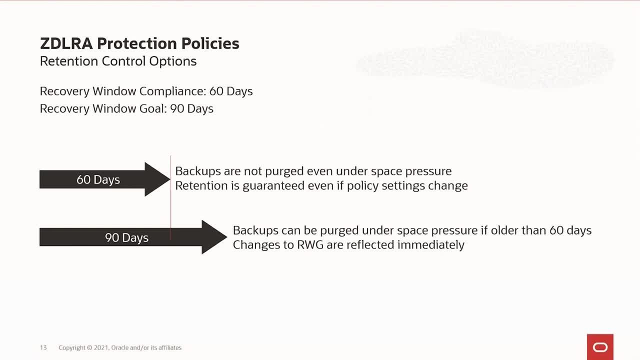 Again. so, as you can see on the screen, so you have recovery window compliance, which is defined for 60 days. So you have window goal: 90 days. so that's your typical retention And, as you can see, for the 60 days within 60 days, backups are not first. 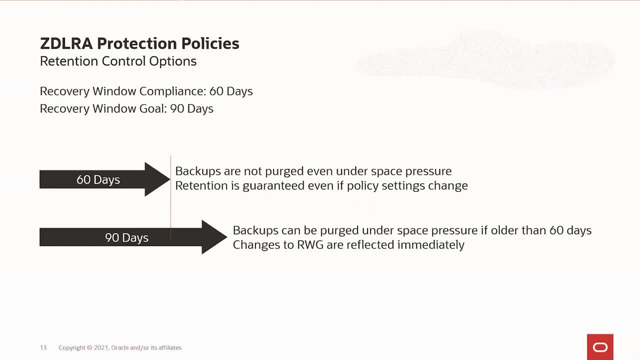 given under pressure On the day 61 and on, backups can be first and you can get the space pressure relief for all the data that are going to be older than 60 days And again, this basically just gives you just a little bit of clarity and a sense of understanding of how you can manage. 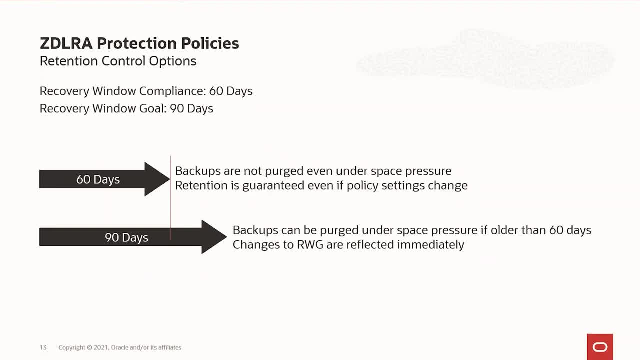 a protection policies going forward specifically related to the existence of the compliance regulated environments. The third window on top, which is the recovery window, SBT, and, as you can see, it's set for 365 days. It is controlled by the ROH, capital confirmation, but again the normal approach after one year. 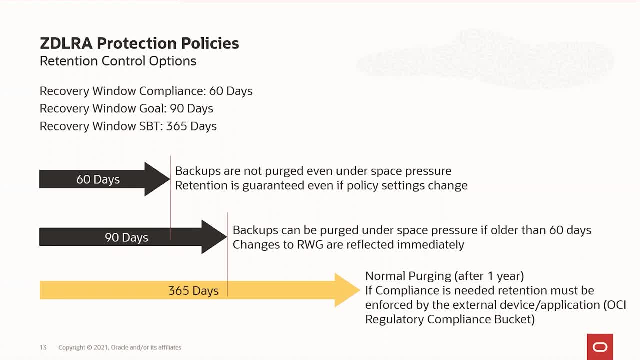 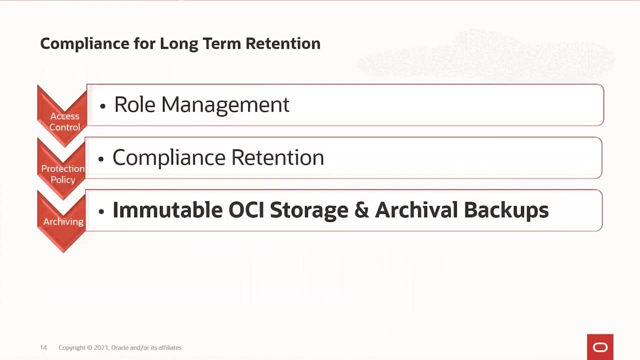 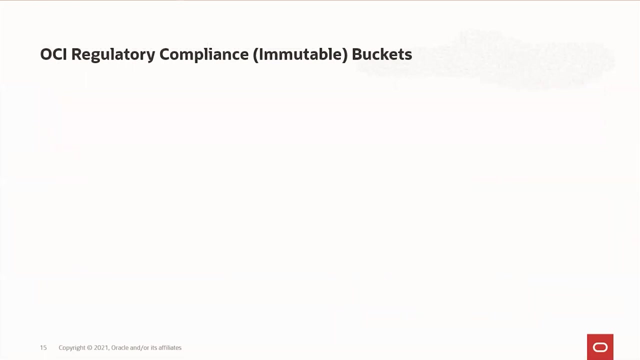 if compliance is needed, and so retention might be enforced on the archive tier, This is going to be enforced by the three share device rather, or cloud services rather than anything else. So let's talk about next important chapter: immutable OCI storage and dark cable backups. This one is targeting, again, the complete deployment of the regulatory compliance. 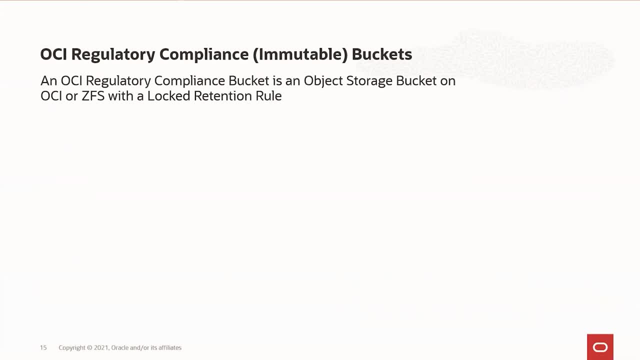 immutable environments. So I already mentioned that there are OCI share compliance buckets that can be deployed in the object storage buckets on the OCI or ZFS, and it also requires a so-called locked retention rule. So this is how it looks on the screen As 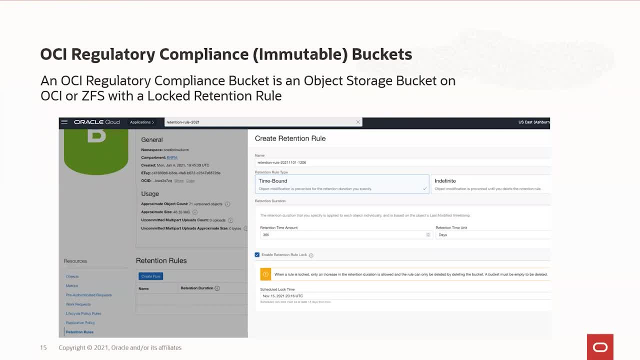 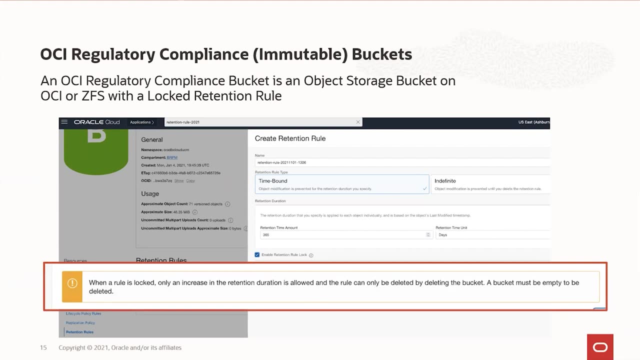 you can see, this is the OCI panel, the Oracle Cloud panel services, And so when you create the retention rule for the compliance bucket, you can enable this rule and then you can get a message that this rule is locked. And the rule is locked, only an increase in the retention. 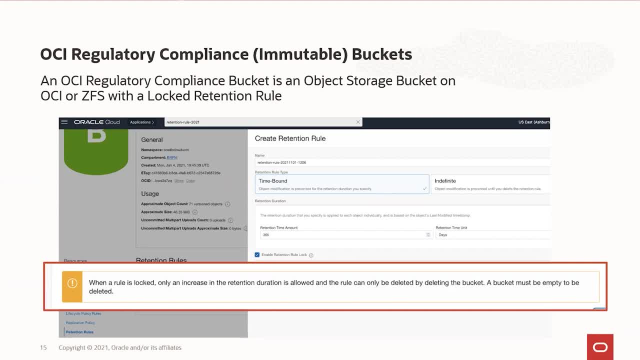 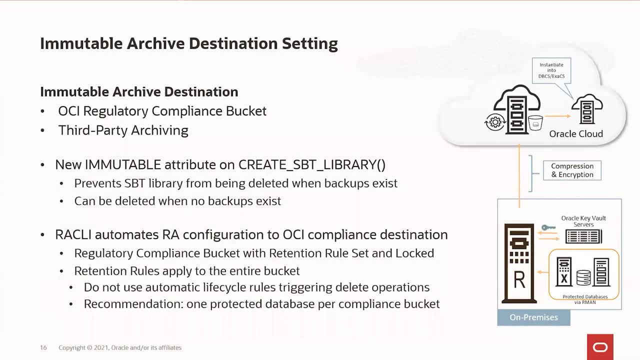 duration that allows this rule. So bottom line, it's going to be delete, so it's going to be outwards, it can be only increased. So from the immutable archived destination settings on the recovery appliance sites. there are a set of new attributes that are related to the SBT. 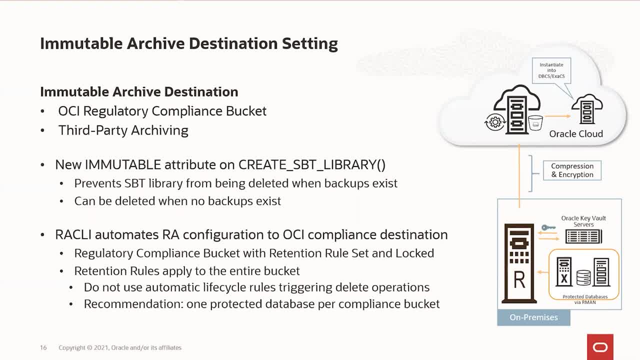 So, as you can see, there's a new immutable attribute that belongs to the create SBT library in the API. And what does it prevent SBT library from being deleted when backup exists? If there are no backups on the array side, bucket can be deleted, but not before you're going to stop all the backup activities on the recovery. 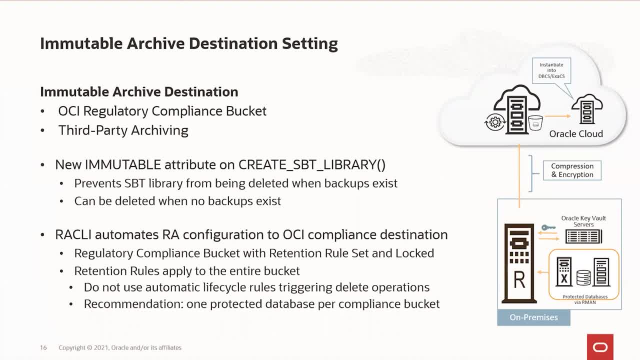 plan side, The array CLI showed me some configuration for the OCI compliance destination And it's basically just make sure that a compliance bucket with retention rule is set and locked, because that actually prevents from breaking any data. So you're going to get error message if you're going to attempt to delete. 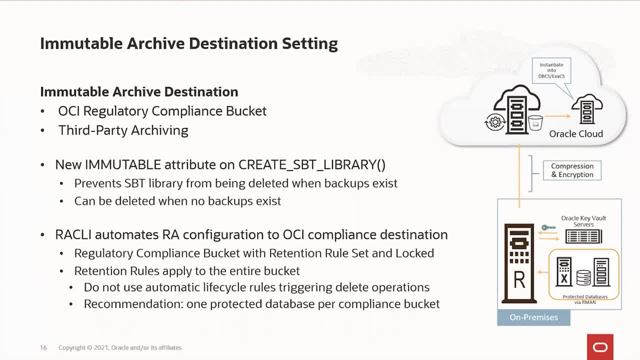 anything in the archive tier, whether it's going to be OCI clouds or it's going to be ZFS. The only thing that's worth mentioning is that the operations related to the archiving tier with the OCI clouds or ZFS are not going to be exposed to the automatic 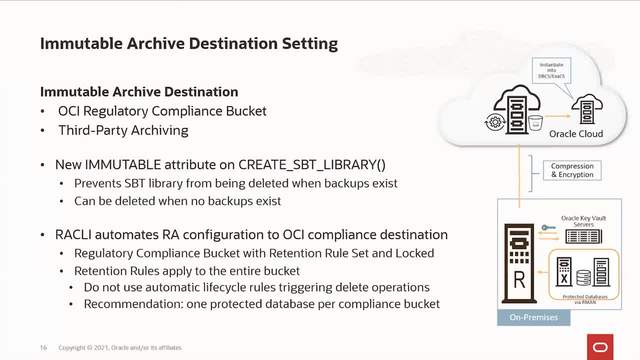 lifecycle rules, because otherwise you're going to destroy your own compliance, obviously because data are going to start expiring on the outside of the compliance regulations requirements that you might face. And so the second one is one: protect Davis for compliance bucket, because you cannot mix and match in different retention periods in the same bucket, So it just makes 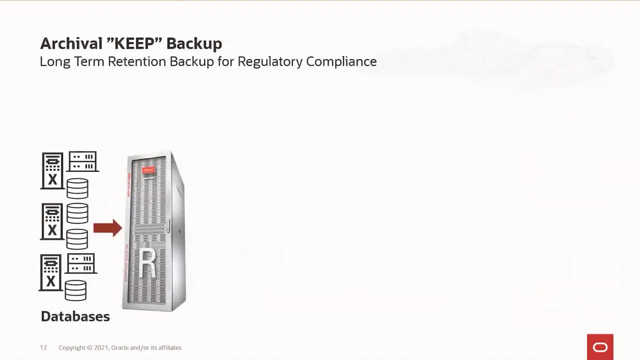 common sense. So let's take a look at the little visual aids in the sense of long-term retention backup For the regular compliance. So you have your databases, And so then you have create our backup, And so the requirement is to keep this archival backup for seven years. So 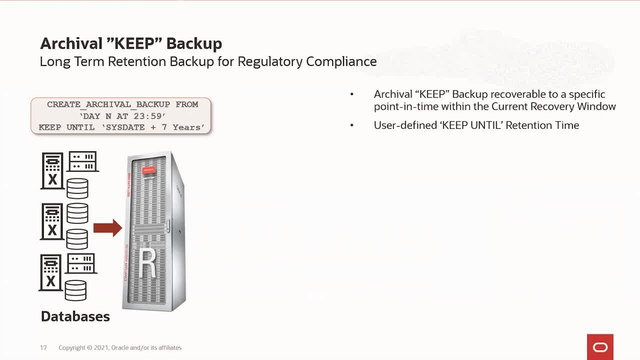 get back up recoverable to a specific point in time, User defined keep on retention time, just all the usual stuff. The only difference between the usual operations for the archive with keep factor is capabilities of the recovery plans to create virtual synthetics out of the transactional data. 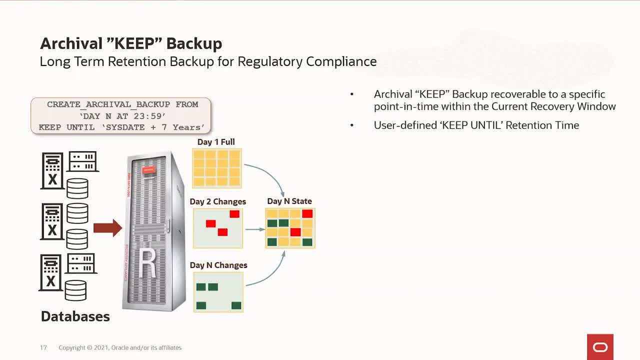 And what it does. that basically offloads all the heavy weight lifting to the recovery appliance side, therefore easing up the overheads on the production environment. So, as you can see, our ratio generates a new image And then it adds logs to recover to the day. 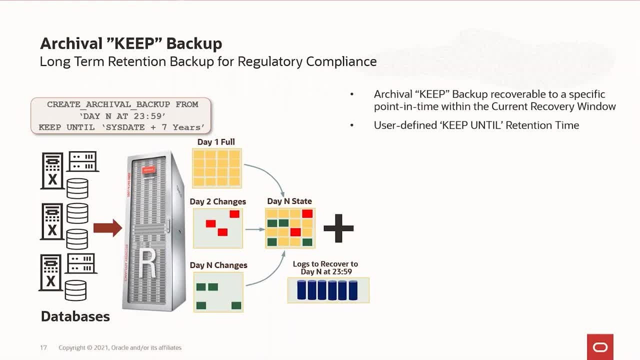 end. So let's say specific time step, it's 2359, close to midnight, And so then it basically generates a complete archive keep image to be shipped out from the recovery plants, And so then it can go to tape ZFS or cloud destination, just like we discussed on the previous slides. 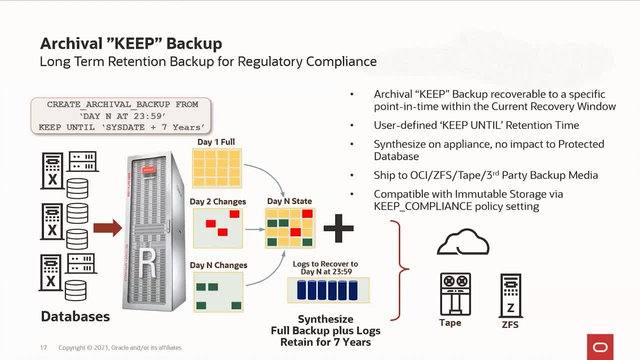 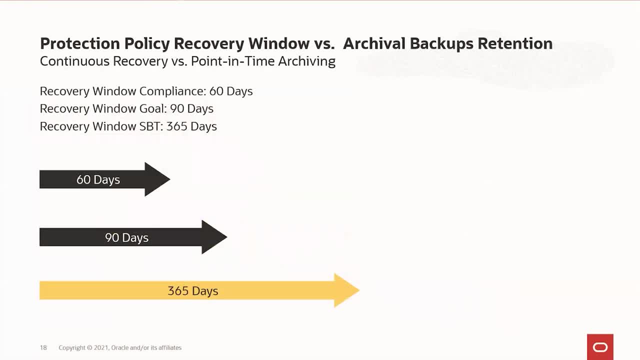 The last factor, it's pretty important that it is compatible with immutable storage keep compliance policy settings. So just elaborate a little bit from the differences between the protection policy recover window versus our cover backup potential. So we had 16-19- 365 days. 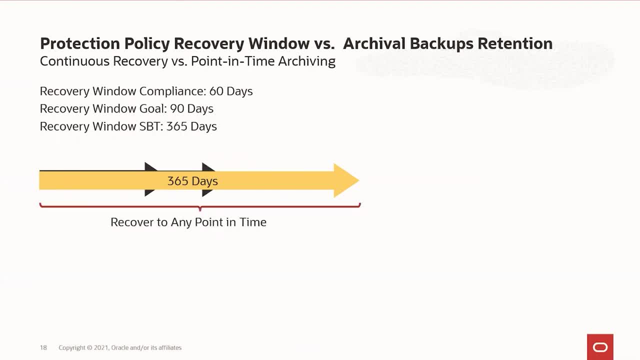 All these tiers of the protection allows you still to have recovery to any point of time. The inhale keeper archive, though, doesn't provide this type of the simmer. it is specific points in time recovery. So RPO recovery point objective can be only accomplished for the specific time step. 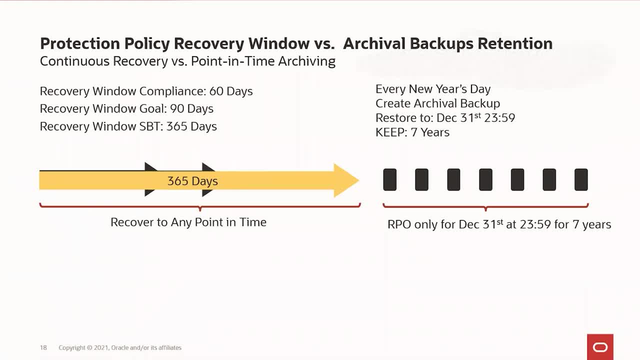 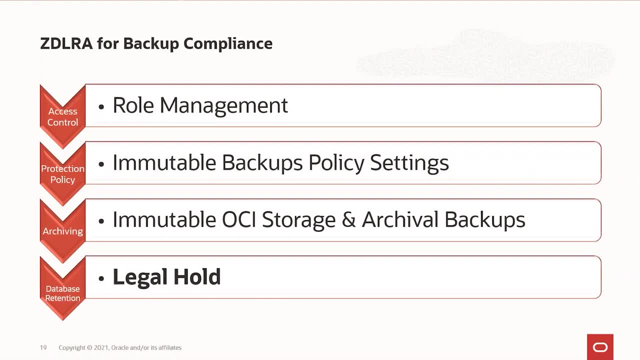 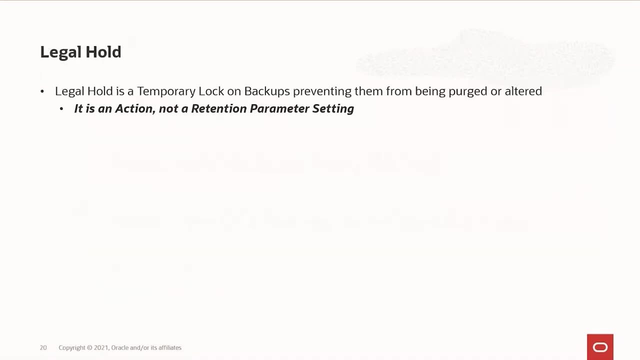 that is associated with this KIPP archival Legal holds a little bit unique flavor of the kind of regulatory compliance but it is oftentimes requires, And what is really important- to understand, that the legal hold is fairly unique flavor of the compliance window management. 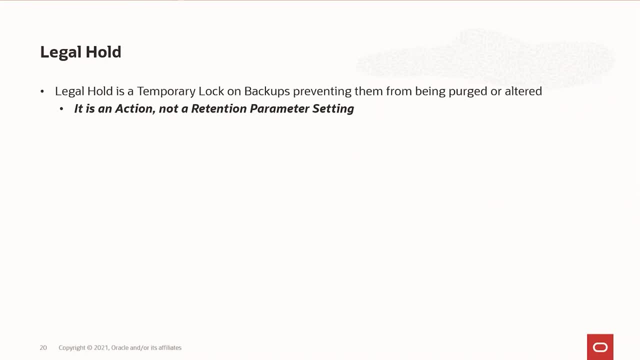 Oftentimes legal holds creates a perception that it's actually related to the retention management, but essentially it's not. It is an action. It is not exactly a retention parameter setting. And why it is an action? Because legal departments, let's say they want to do some heavy 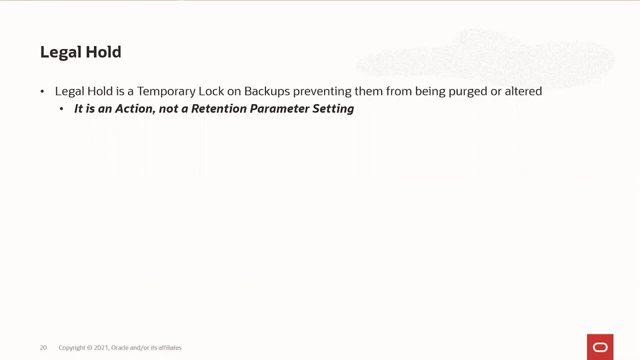 research within the backup and archive data, And so they come to you as the environment owner And so they say that, listen, we need to hold artifacts XYZ by the specific criteria And until we're going to be done with the legal discovery process. 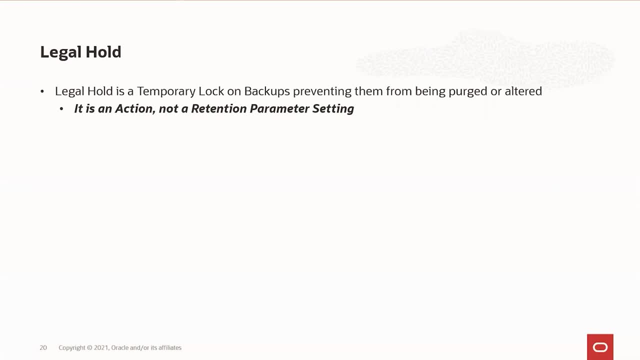 these artifacts can be touched. So therefore it is both action, in a sense of how it's being imposed and how it's being managed, But at the same time it is relevant to the retention parameter settings Because, for example, we go hold might list that year. 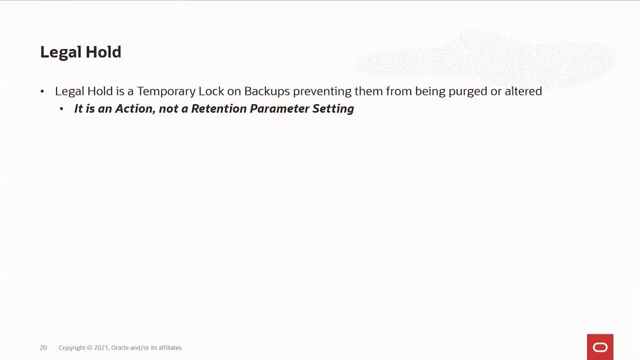 And you aren't, as of the environment owner on light, have specific requirements that you have to keep your data on livestream 30 days. So this one year of the legal hold action is basically super scenic and and that is related to the retention management, 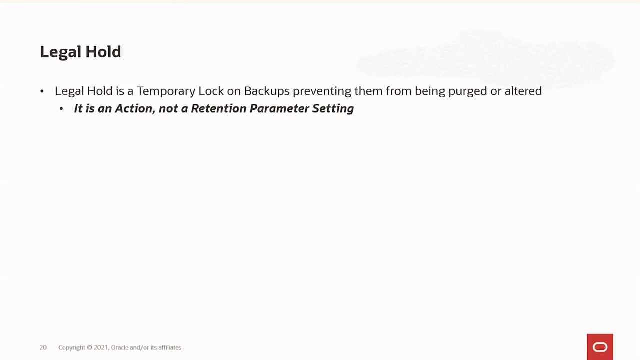 And so this was a little of insert to balls as an action, but at the same time just to have a clarity of the understanding of what might be implications in a sense of the overall data lifecycle and so retention management. So there's a new compliance hold. 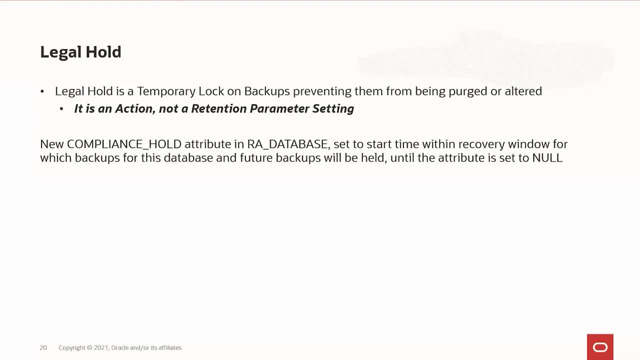 attribute which is set on the array database, and what it does? it basically starts them within the recovery window, for which backups or database will be held until the attribute of the compliance hold is set to null. So back to my previous points. these are the actionable items rather than 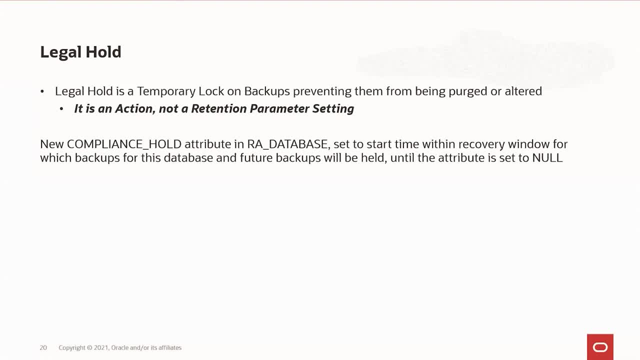 retention setting. As you can see, you set up on the environment compliance hold and then you set it to be released with a null Again, it can only apply to the array local storage because obviously we cannot impose our settings on anything outside of the recovery appliance environment. 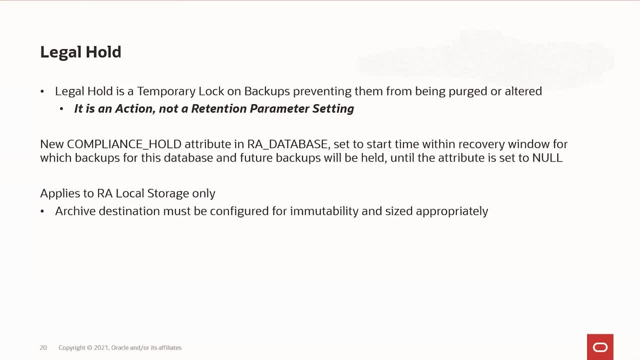 So archive destination must be configured for the immutability and size properly if you do expect something like that happening in your IT environment. So you set keep compliance protection policy to yes, and so then you can configure legal hold for the OLCI storage destination. There are some specific requirements for the OLCI buckets. It must be: 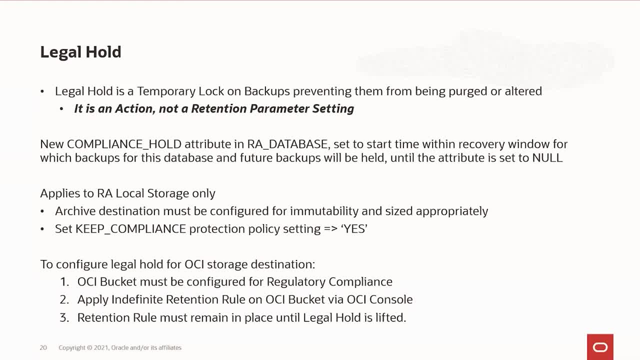 configured for the regulatory compliance. You can apply indefinite retention rule on the OLCI buckets with the OLCI console and retention rule must be remained in place until legal hold is lifted. Like I said, it's just all common sense requirements. As you can see, it cannot be basically just. 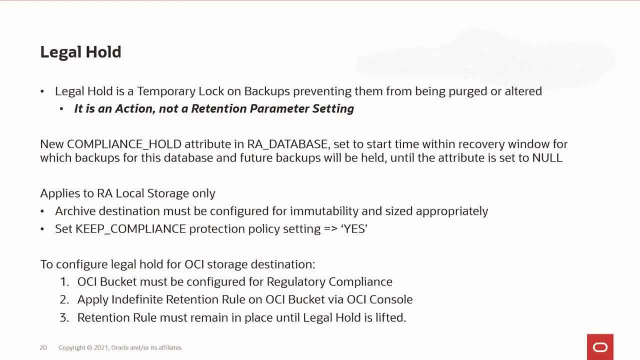 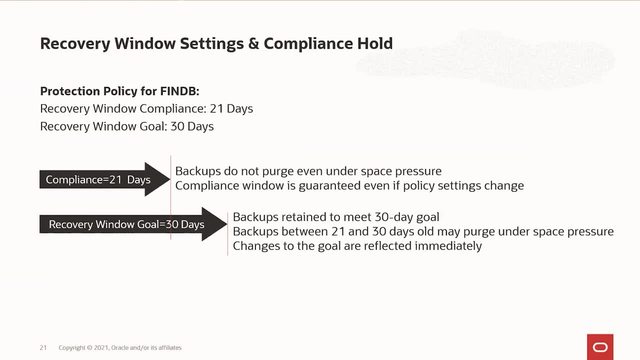 carried over from the primary to the backup, to the archiving tiers. Um, just to make sure that so we are on the same page and how actually the legal holds actions is going to be applicable to the overall compliance environment, and so you have compliance with 21 days. nothing can be perched. Then you have to apply normally every civilian to these. inspection days which were 부분 for maintenance work. But, as you know, the original IT environment only has a set manifest California, or a set I wore, environment- areas and standard. You screen this in the extension of a census paper which I registered. this presentation at 35條ht. 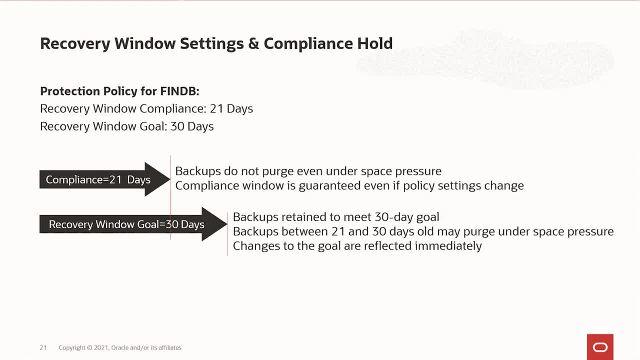 then you have a recovery window go for 30 days or so. your data has 21 day can be purged. Nevertheless, if you impose compliance hold, it basically cuts across both compliance window and usual window go. So anything starting from the specific points on is going to be affecting every. 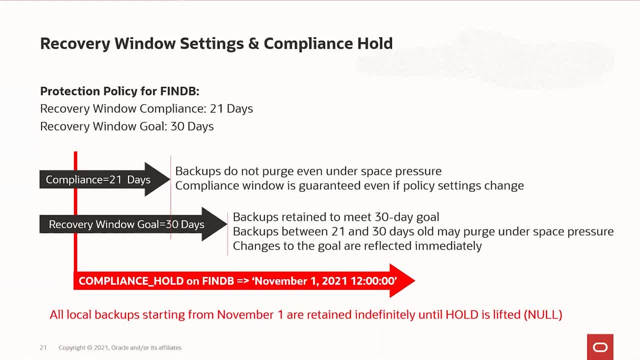 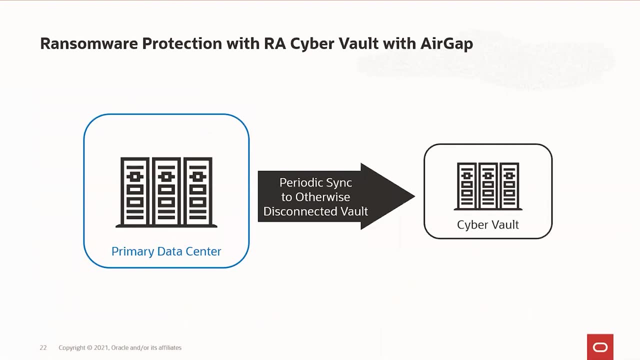 backup data that are going to be resigning on the recovery appliance And, yet again, they're going to be retained indefinitely, until the hold is going to be lifted by setting to be parameter null. So just to recap the journey for the overall immutable environment. 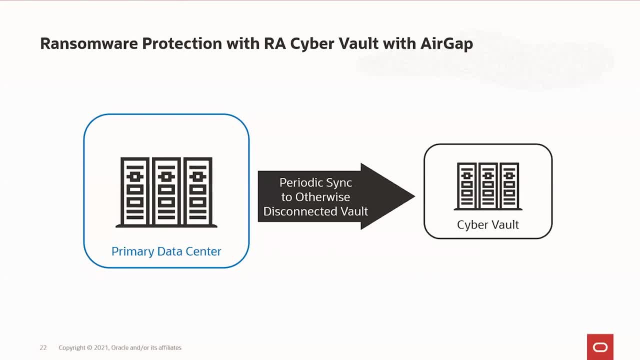 started with the recovery appliance providing with unique capabilities for the ransomware protection with recovery appliance, cyber vault with air gap settings. So there's not the special flavor though for recovery appliance, It's actually the just a basic configuration over the receiving recovery appliance. What is unique? 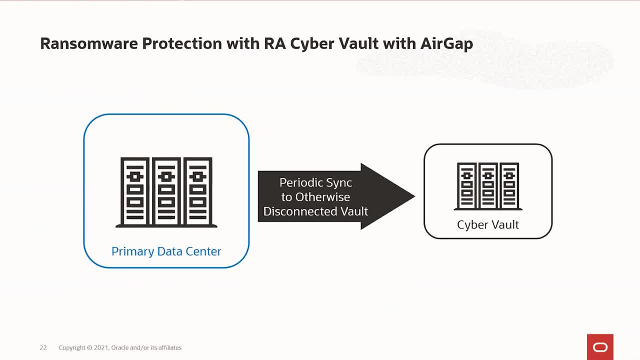 for the several world configuration is that we do not have a persistent connection between the primary data center asking for data to be synchronized. So there's just yet another layer of the defense, ensuring that if you have some sort of the bridge of the overall accessibility. 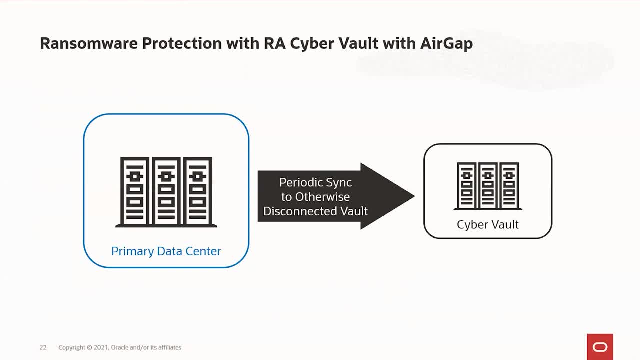 to the backup environment, you're still going to be most likely protected because Cyber Vault is going to be initiating the reverse request for the replication on the random schedule. So most likely raw vectors are not going to be able to identify when actually a connection is. 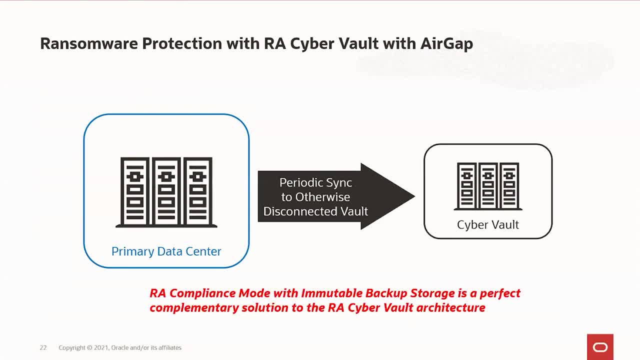 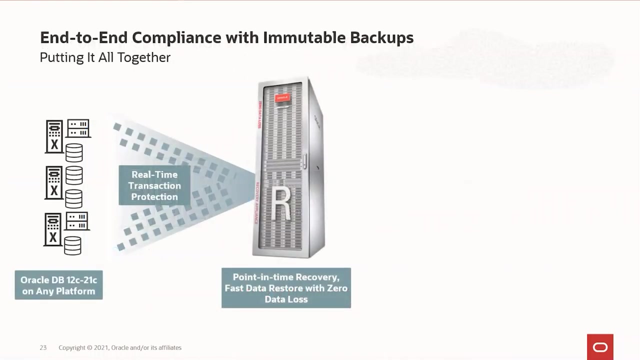 going to be occurring between the Cyber Vault and the primary data center. So why it is important? because, if you will take everything that we discussed until now, it is pretty evident that recovery appliance compliance mode with immutable backup storage is a complementary solution to the RA Cyber Vault architecture overall. So from the putting it all together in a sense of the 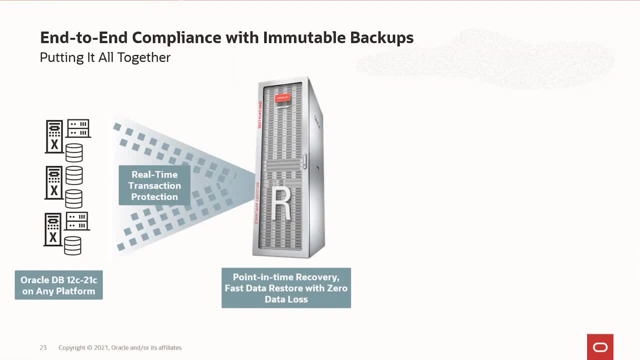 operational availability and management. so you have your Oracle databases. So, as you know, recovery appliance supporting pretty much all the current releases from 12C to 21C, on any platform. You have real-time transaction protection. of course You have point-of-time recovery. 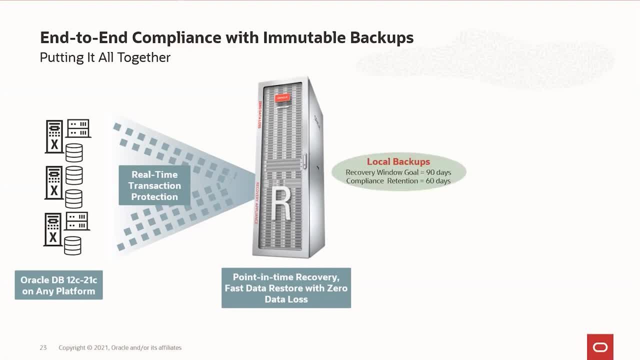 provided by the recovery appliance And, from the management standpoint, if you can imagine, like set of policies, this is basically just how it actually works overall. So you have local backups. with the recovery window called the 90 days, you can set your compliance. 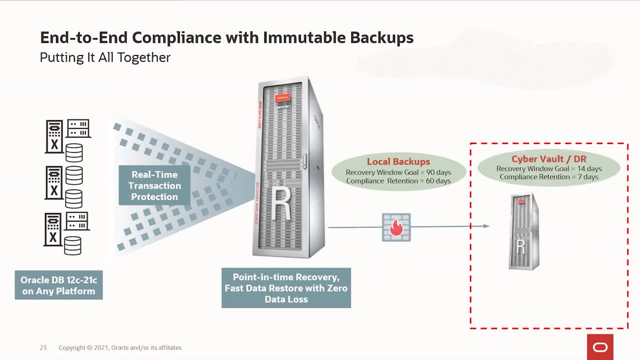 regulation to 60 days. Then there's going to be a fan out for the replication to the Cyber Vault disaster recovery appliance. You set another policy for the recovery window go 14 days, compliance retention seven days, Then you have your archiving tier, like in this particular case. 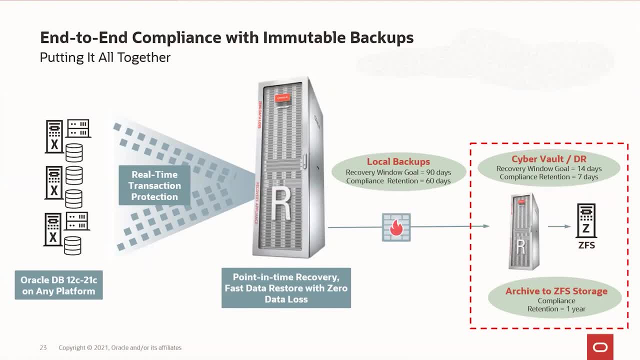 on the slide. as you can see, this is archived to ZFS storage with the sets for the compliance retention one year And obviously, if they fan out, directly to the object storage with yet another compliance retention, let's say for seven years. 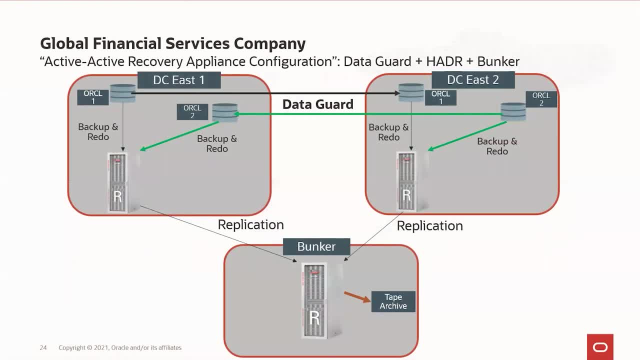 Just to give you some sort of real-life example. so this is the policy for the Global Financial Services Company. They have two data centers, DC-East-1, DC-East-2, and then they have a bunker for the deep archive and tape out. 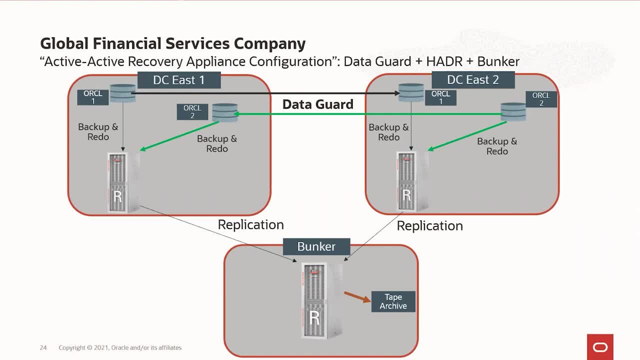 As you know from the best practices, they follow TMA advisories so they set two data centers of high availability with Data Guard, So you have production and you have a secondary infrastructure as of the call standby, and then you have two recovery appliances acting as the 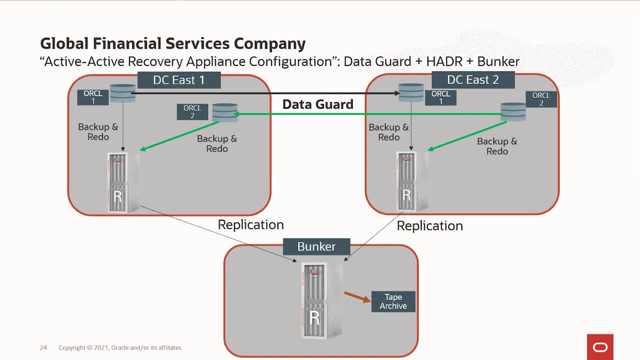 backup. This is just pretty unique to the overall data protection offering by Oracle. If you take a look at the competition, it's virtually impossible to accomplish in one shot high availability, disaster recovery and backup practices. It typically requires a different set of tools. 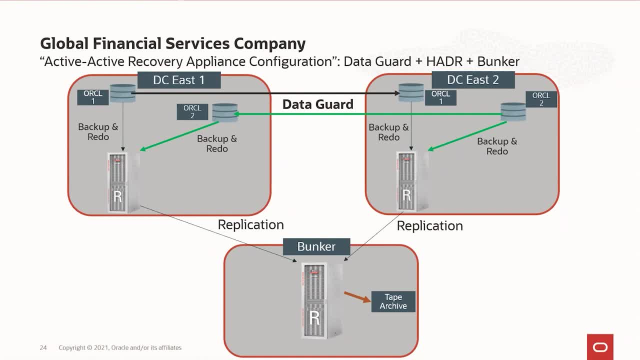 and they are not really coordinated or anyhow integrated between them. In our case, this is directly opposite. We can provide all these qualities and we can ensure that your environment is practically bulletproof. So what is new here is the fan out from the backup. 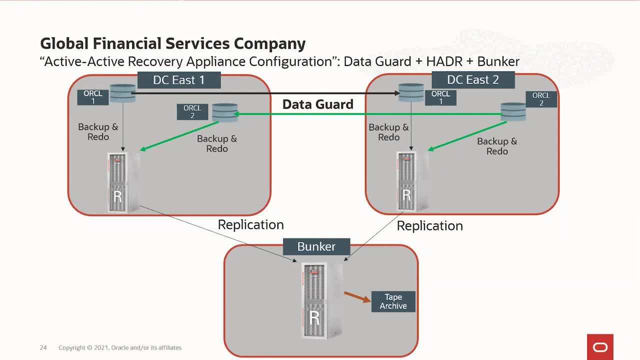 appliances on the DC1, DC2, going to the bunker with specific retention requirements, And then obviously the TAPA archive, which is the archiving tier, And then obviously it's going to be carrying out a little bit different set of the requirements for the archive, But from the 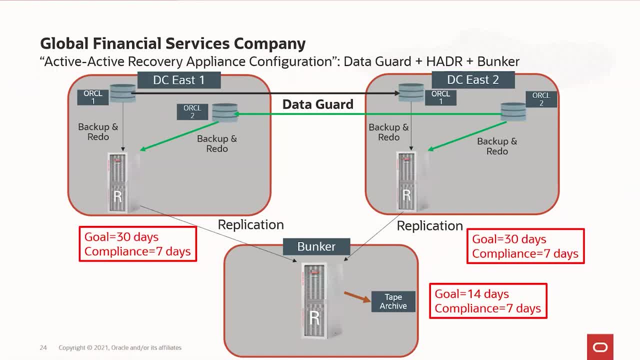 management standpoint. so you have go: 30 days compliance, seven days on the primary. You have exactly identical requirements on the primary. You have exactly identical requirements on the primary. You have exactly identical requirements on the primary. You have exactly identical settings for the secondary. DC is tuned with the same goal: 30 days compliance, seven days And. 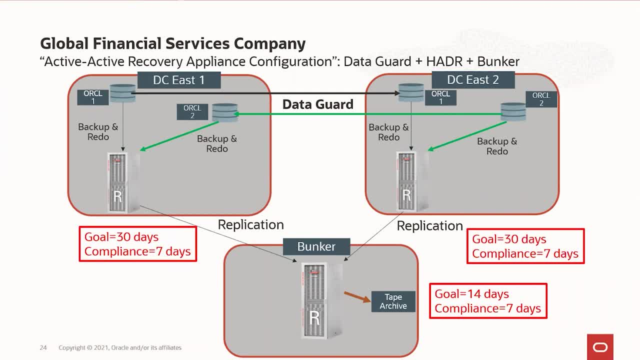 then you have separate policy for the seven days and compliance, seven days on the bunker one, And then you have TAPA out And obviously in this particular case it's a warm device, right one. so with the compliances, So in this particular case, 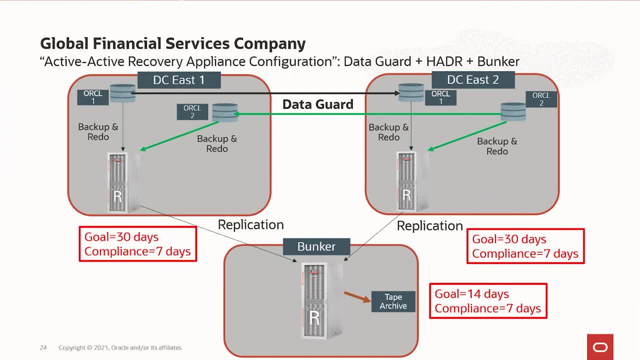 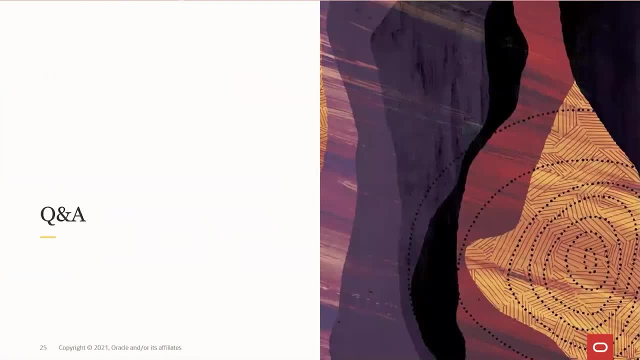 financial services are most likely is going to be somewhere between seven years and so in infinity. That's the wrap. That's all I have to tell you about the latest and greatest. so by the recovery appliance team with the new release 21.1 and we can move on to Q&A. see what's happening. 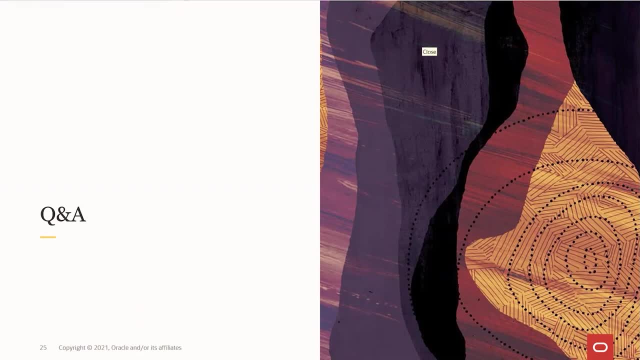 Hey Alex, Thanks for that presentation. I'm going to add in the chat the link to our ransomware 21.1 new features blog, so please take a look at this. I'm just going to add in there. It's about add that here. thank you, tim. 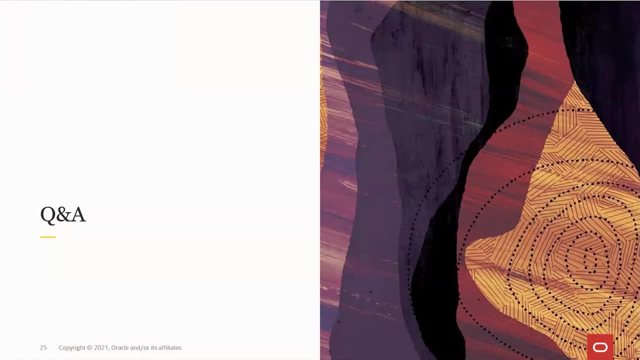 so i have a few questions here that weren't already answered, but i think well, distribution for the powerpoint: everything is going to be available on the website, as always, both recording and powerpoint. the retention periods- if a question, if any retention period can be modified, post backup. 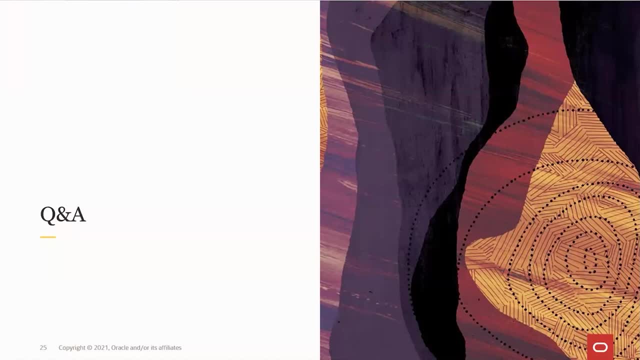 so again, if you do not want to compromise your environments, and then most likely you're going to be imposing compliance on the top of the backup protection management. so the answer is absolutely not, because otherwise you basically breach the compliance and so obviously you're going to be. 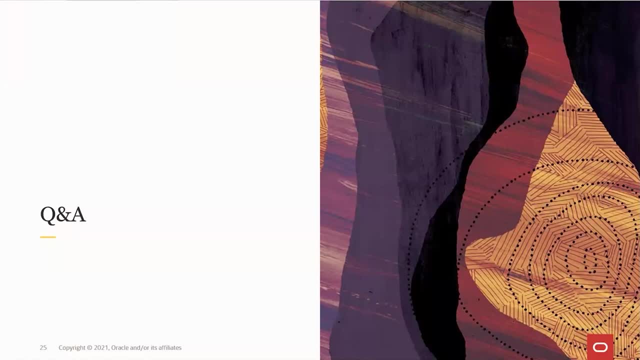 out of the regulations. do we have any other questions? tim, i'm not seeing anything noted. kelly already answered the one question about how retention works with compliance and if it can be altered. so yeah, so that that's a good point that once a compliance retention is set, that retention cannot be reduced for existing backups, right so 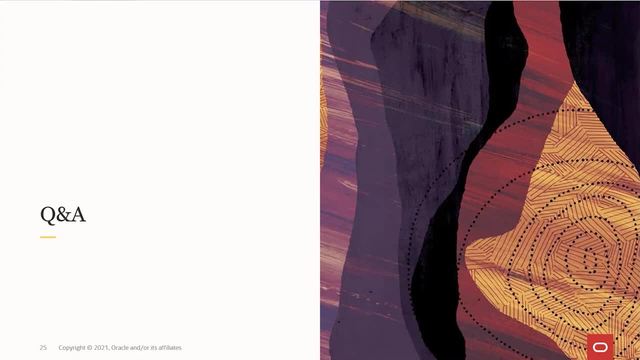 if you do alter that compliance retention, it will. it will only take effect for new backups after that point. thank you, tim. let's give it a couple more minutes, if you know gets any new questions. well, i don't see anything new in the queue, so, um, thank you again. i really appreciate your time. 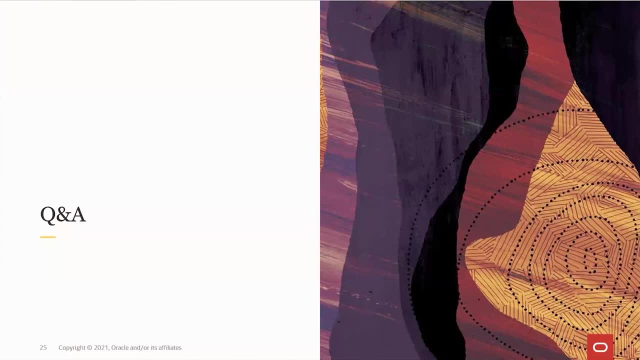 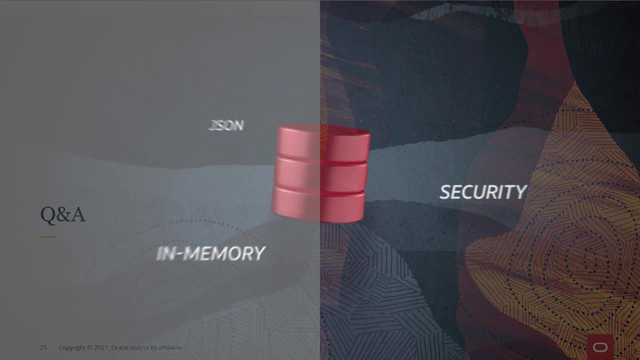 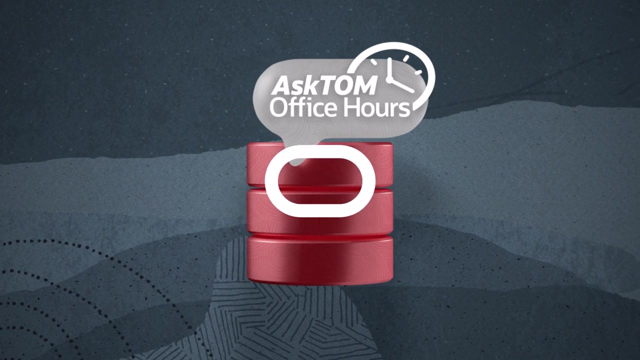 and your availability for this session. i hope it was helpful and if you have any following questions, so please feel free to reach out to your support or your sales team. thank you again. happy friday, have a great weekend. i'll see you later you.